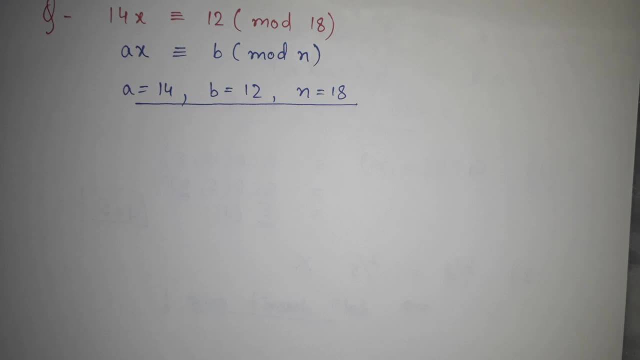 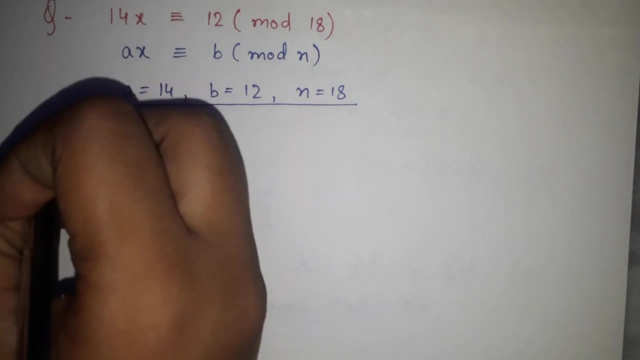 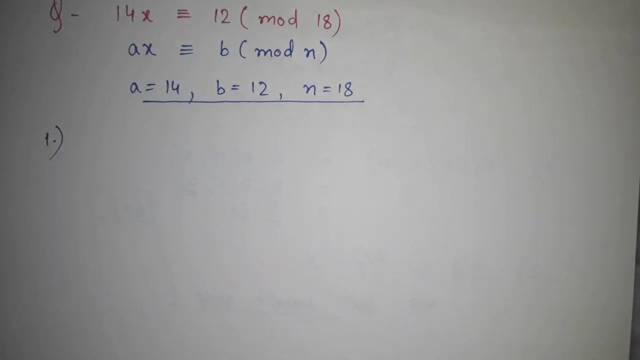 You can take a snapshot Or you can note it down somewhere. It will be easier for you to understand. Okay, So the first step we were having was finding the GCD of a and n. First step, let me write it here for you. In the first step, what we will do is we will find out the value of GCD. 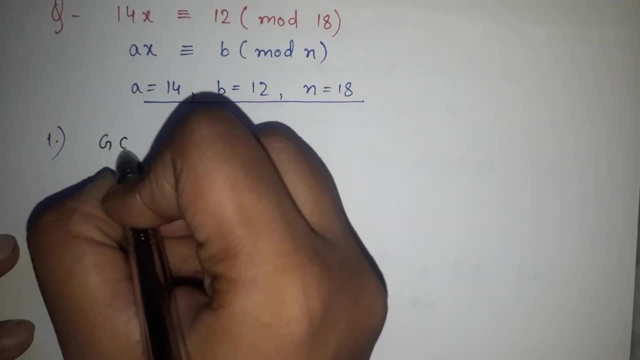 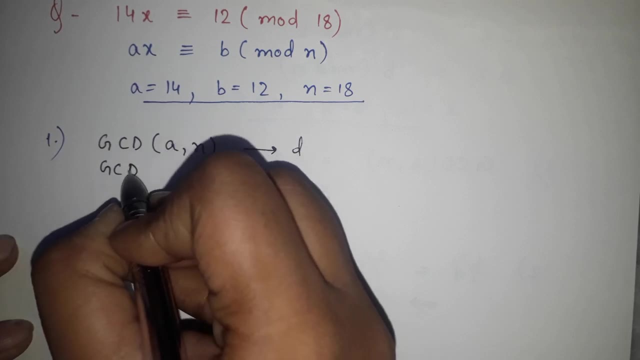 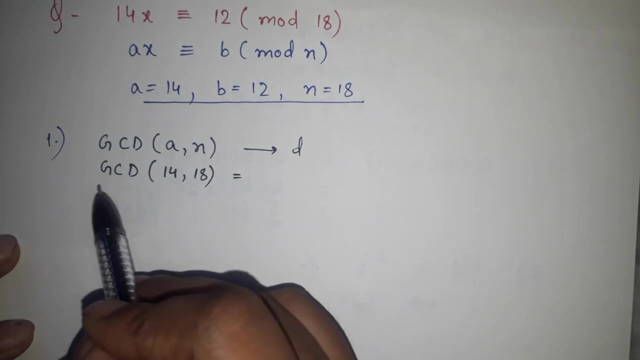 of a n, GCD of a n, and we will, whatever we will get, we will name it as d. So here we will have to find the GCD of 14 comma n, that is, 18.. 14 comma 18.. You can find GCD for with the help of various methods. 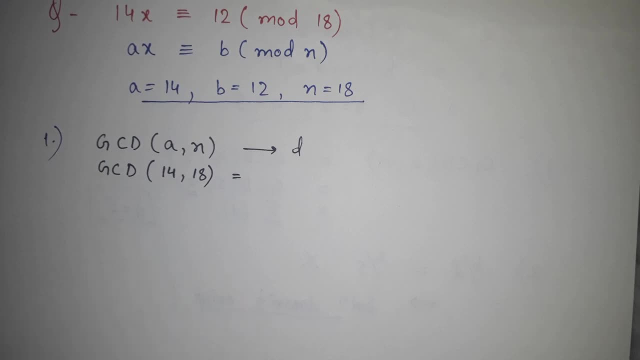 We are having Euclidean method, extended Euclidean method. you can find out directly. Okay, So you can choose your own way. But here the numbers are small: 14 and 18.. So we can directly say that GCD of 14 and 18 is 2. The greatest common divisor that can divide 14 as well. 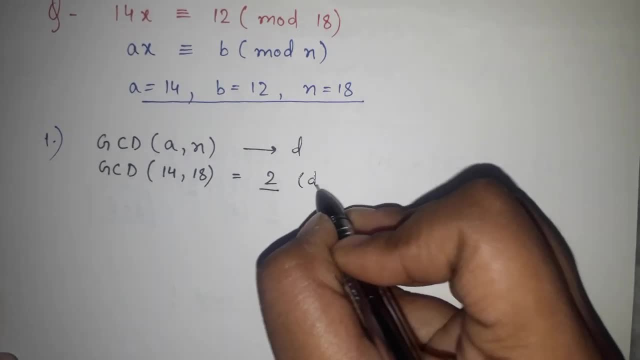 as 18 is 2.. So I got the value of d as 2.. Alright, So we can find out the GCD of a and n. We will find out the GCD of a and n. So we can find out the GCD of a and n. So we can. 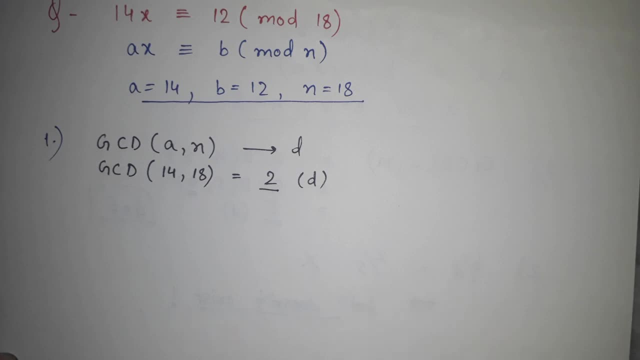 find out the GCD of a and n. Alright, This is my first step. The second step is we have to perform b by d and whatever answer I will get, we can say that if I can by b by d, if I am getting one whole answer, exact answer, I can see that I can say that the solution 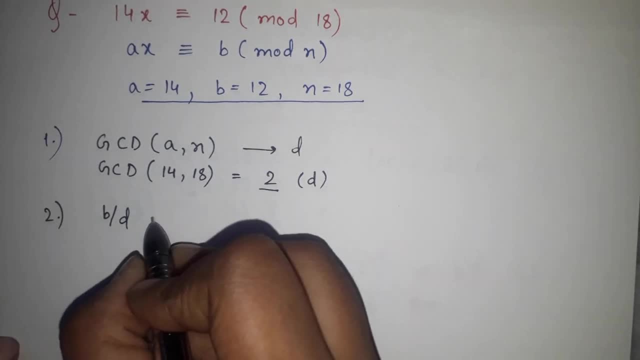 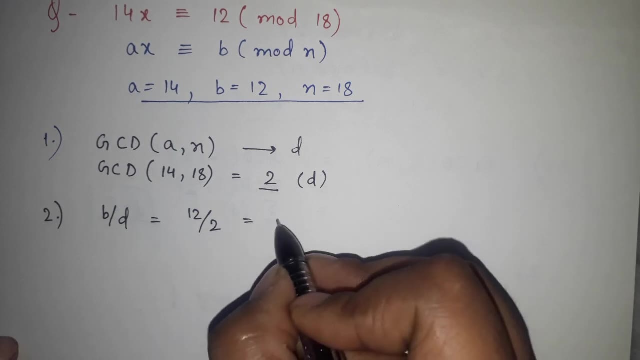 exists, otherwise solution does not exist. So b by d is equal to: in my case b is 12, d, we have find out as 2.. So 12 divided by 2, we are getting 6.. So we can say that this is a complete number. it is a complete number, So I can say that. 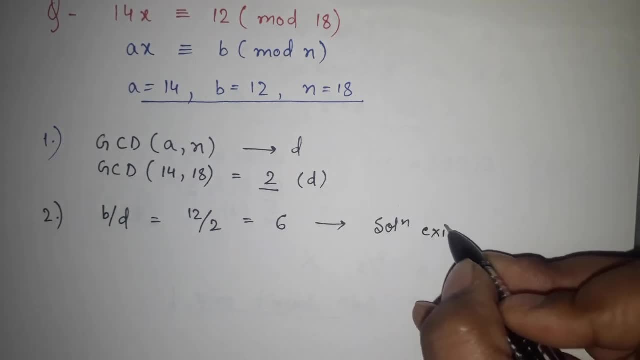 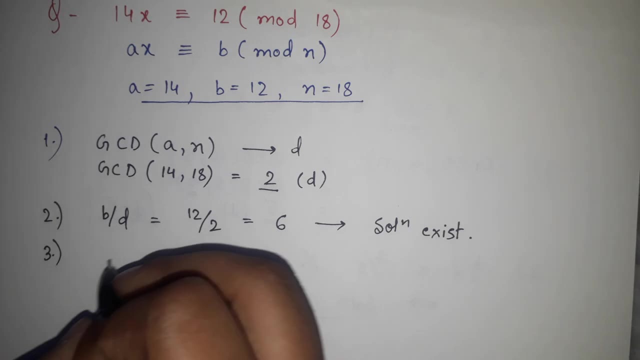 yes, solution does exist. We have found out that solution exists. Now, how many solution exists For that? we are having third step. the formula is d mod n. we will find out d mod n And whatever answer we will get, those many solutions are possible, right Solutions? 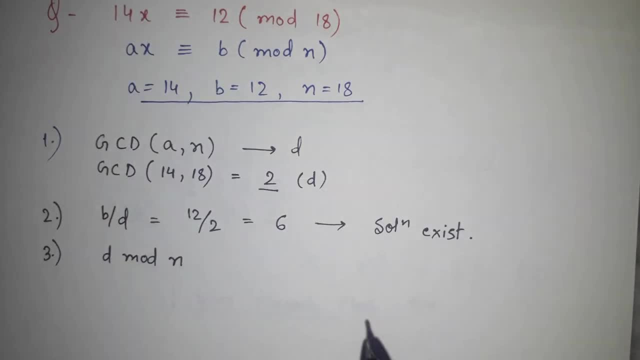 are possible, means those many values of x we can found out. So here d mod n and is equal to 0. So this will be us instead of what. So we get this on. So for the next step, we cannot compute all these. So we can find out the 2 d by d. So I got it. So here is the destroyed. 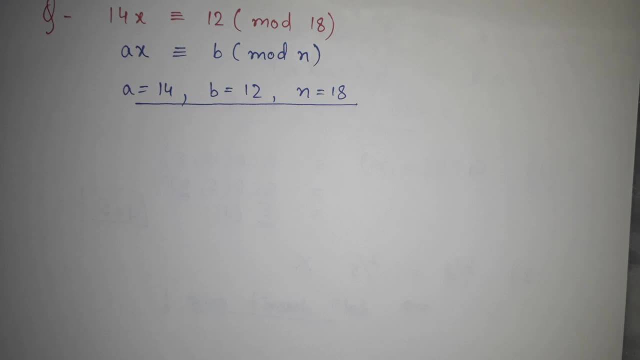 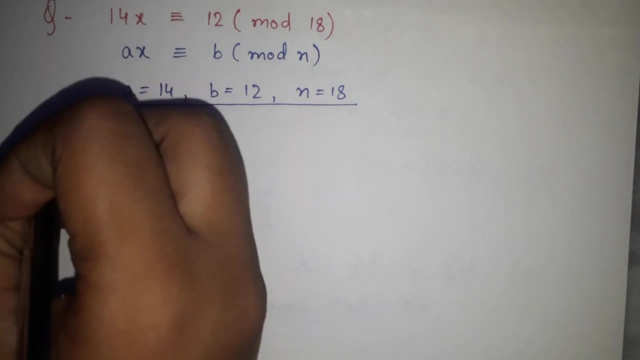 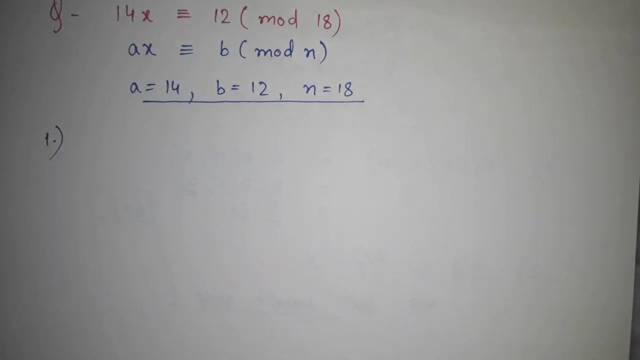 You can take a snapshot Or you can note it down somewhere. It will be easier for you to understand. Okay, So the first step we were having was finding the GCD of a and n. First step, let me write it here for you. In the first step, what we will do is we will find out the value of GCD. 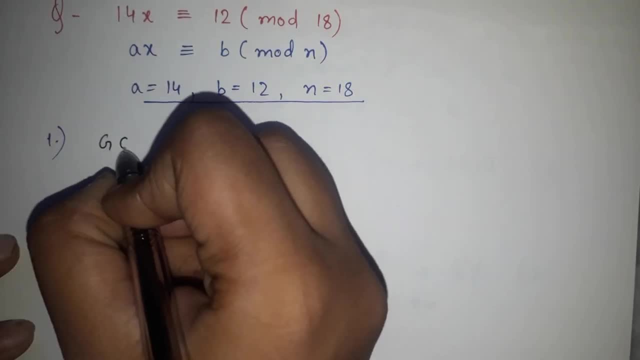 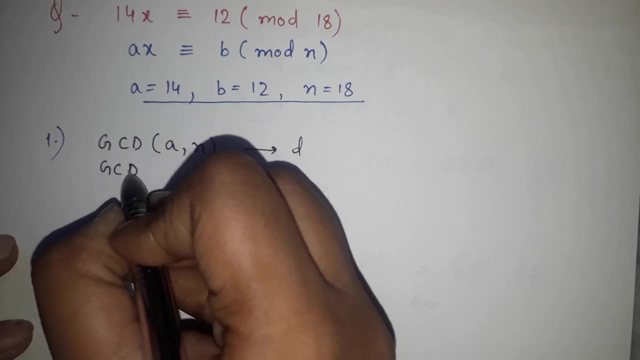 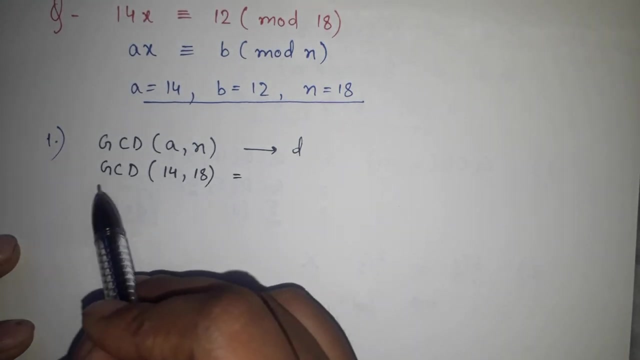 of a n, GCD of a n, and we will, whatever we will get, we will name it as d. So here we will have to find the GCD of 14 comma n, that is, 18.. 14 comma 18.. You can find GCD for with the help of various methods. 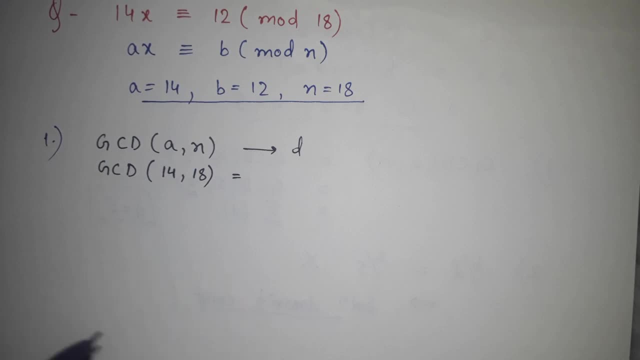 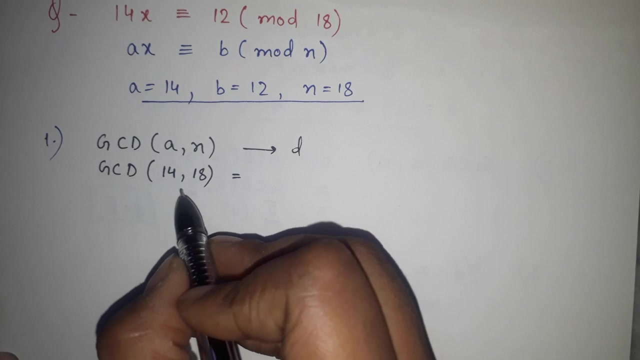 We are having Euclidean method, extended Euclidean method. you can find out directly. Okay, So you can choose your own way. But here the numbers are small: 14 and 18.. So we can directly say that GCD of 14 and 18 is 2. The greatest common divisor that can divide 14 as well. 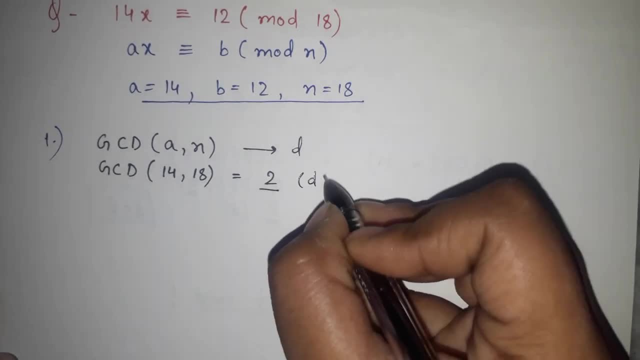 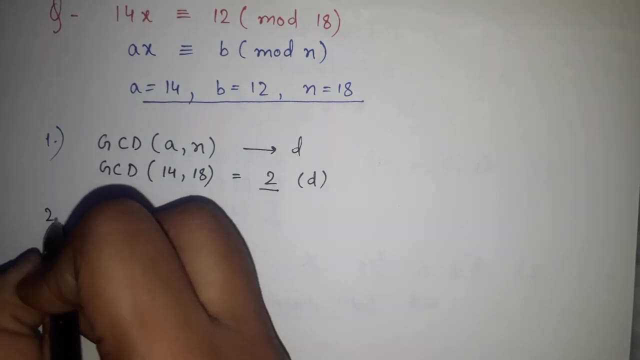 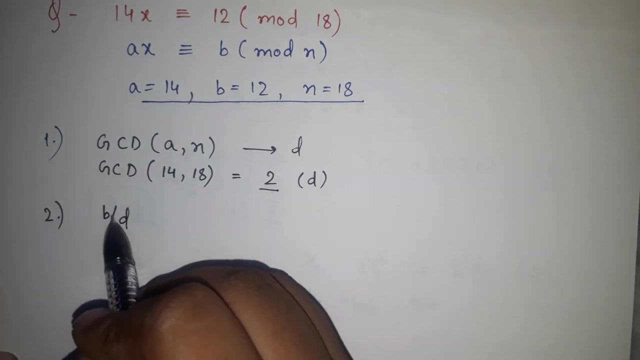 as 18 is 2.. So I got the value of d as 2.. Alright, This is my first step. The second step is we have to perform b by d and whatever answer I will get, we can say that if I can by b by d, if I am getting one whole answer, exact answer. 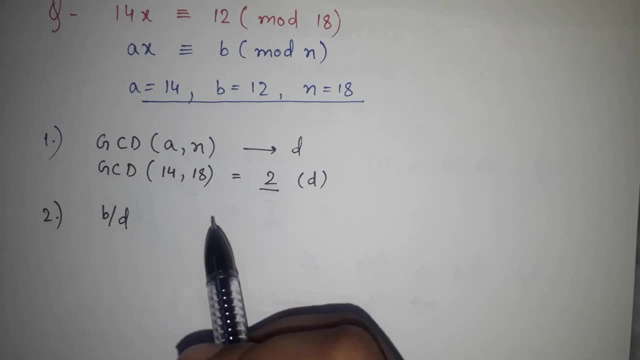 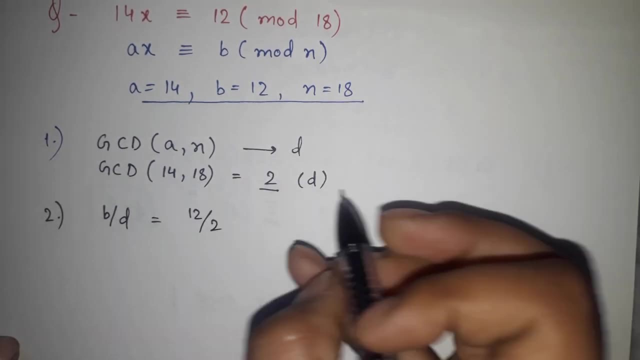 I can say that the solution exists. otherwise solution does not exist. So b by d is equal to. in my case, b is 12, d, we have find out- as 2.. So 12 divided by 2, we are getting 6. It is a complete solution. 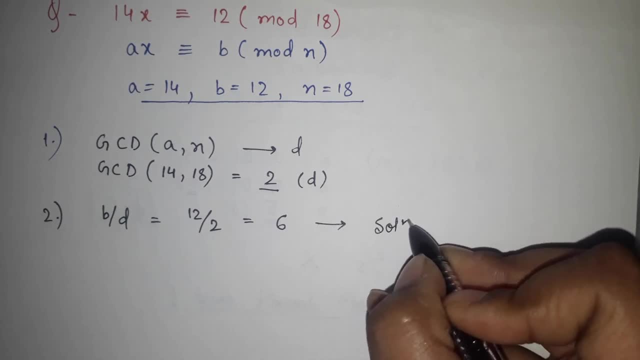 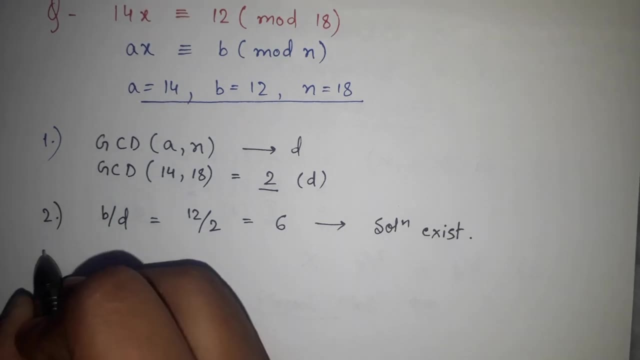 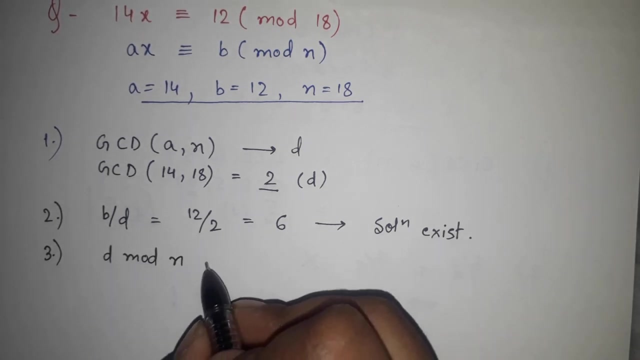 So I can say that yes, solution does exist. We have found out that solution exists. Now, how many solution exist for that? we are having third step. the formula is d mod n. We will find out d mod n and whatever answer we will get, those many solutions are possible, right. 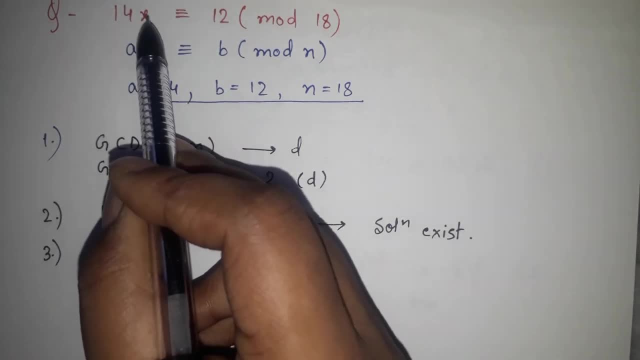 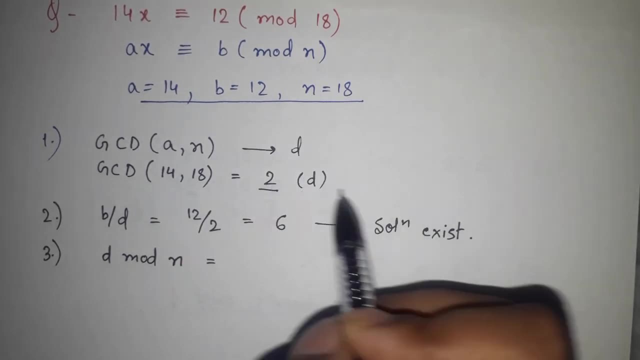 Solutions are possible. means those many values of x we can found out. So here d mod n, that is equal to d mod n. So d mod n is equal to d mod n. So d mod n is equal to d mod n. So d mod n is equal to d is, in our case d is. we have found out d is 2. d mod n n is 18.. 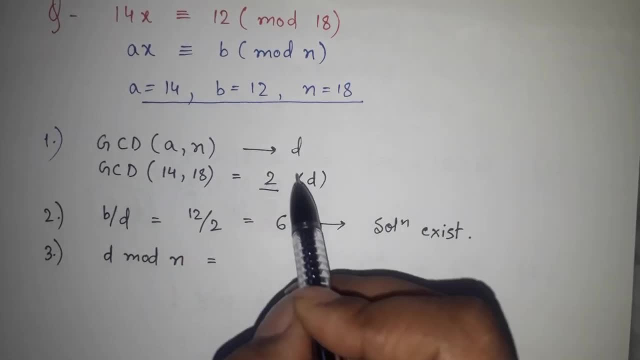 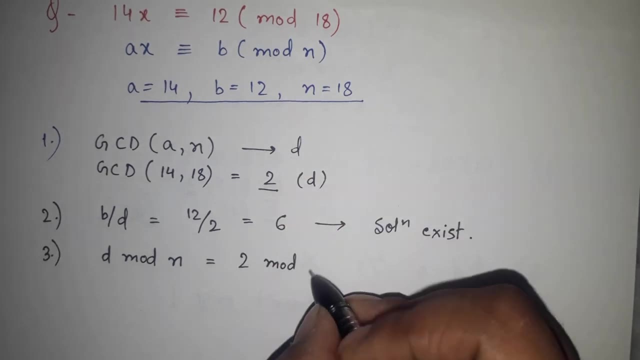 that is equal to d is. in our case, d is. we have found out d is 2, d mod n n is 18, so 2 mod 18,. 2 is a smaller number, so we will get 2 as it is. 2 mod 18 is 2, so I can. 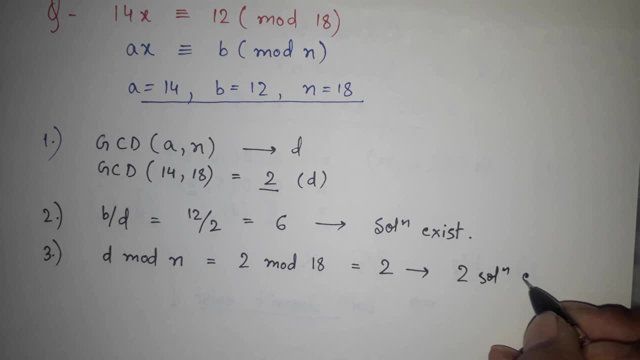 say that 2 solutions exist, 2 solutions. what I mean by 2 solution exist. 2 solution exist means at the end I will get 2 values of x right. so this is my third step. fourth step says that divide both the sides by d. divide both the sides by d, divide both the. 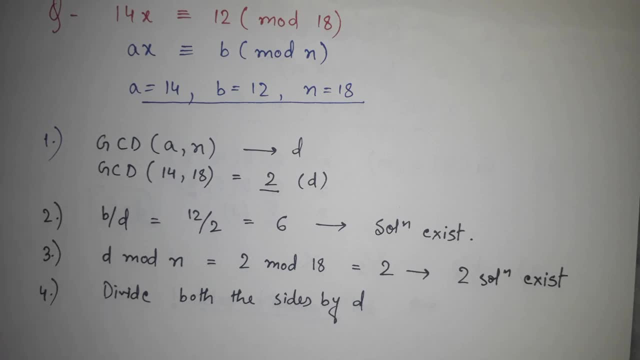 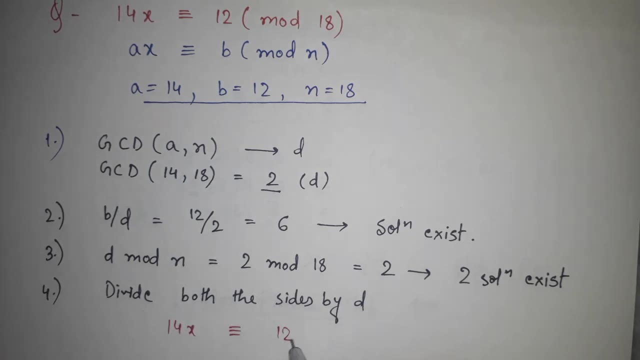 sides by d, so both the sides by d means by default. my equation is my equation. that is already given, so it was 14.. 14x is congruent to 12 mod 18,. right now what I have to do is I have to divide both. 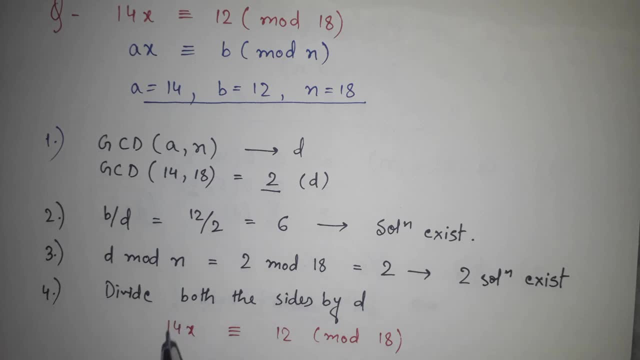 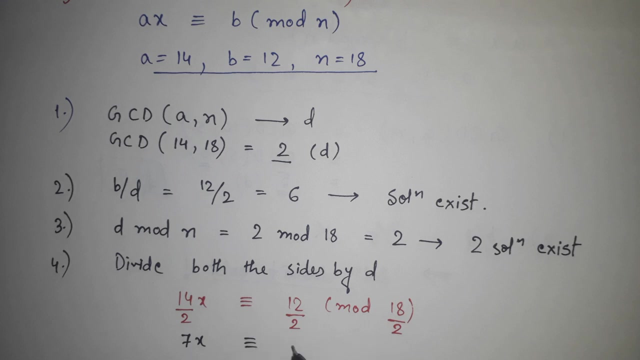 the sides by d. in my case d is 2, so I will divide both the sides, all the numbers, by 2, so dividing them, what I will get is dividing them. I will get. 7x is congruent to 6 mod 9,. 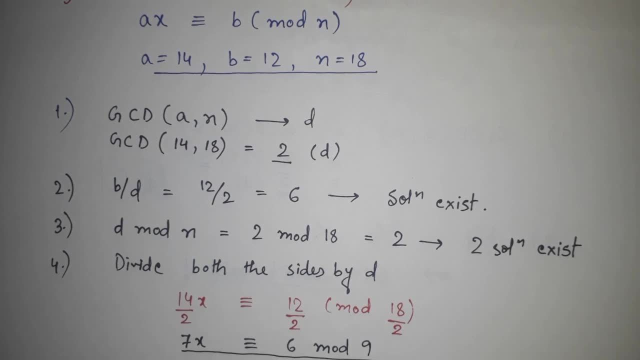 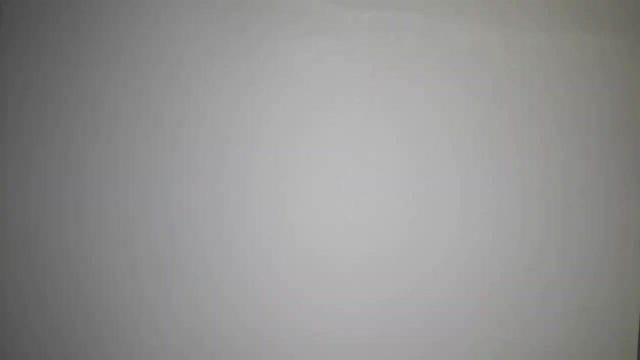 right, I will get this equation that 7x is congruent to 6 mod 9,. now I have got this in the fourth step, so from the fifth step, I will take this equation and I will carry out. this is my, this is my fourth step. then, in the fifth step, what I will do is in the 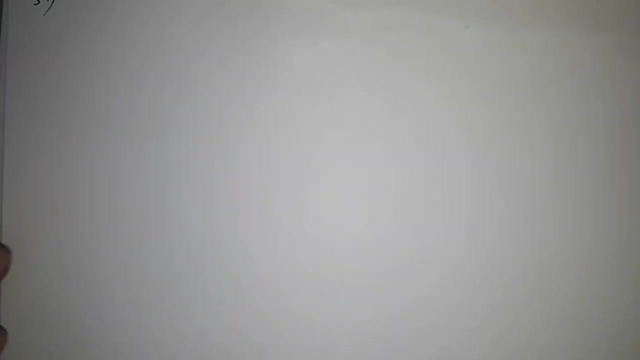 fifth step. in the fifth step, I am having you take those steps, take those steps with you So you can get a clear idea, though I am writing the steps. ok, from here, here up to here. we have done up to the fourth step, dividing both the sides by d. ok, after dividing both. 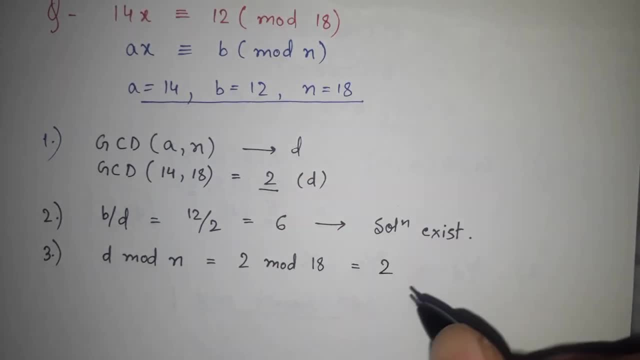 So 2 mod 18.. 2 is a smaller number, So we will get 2 as it is. 2 mod 18 is 2.. So I can say that two solutions exist, Two solutions. what I mean by two solution exist, Two solution. 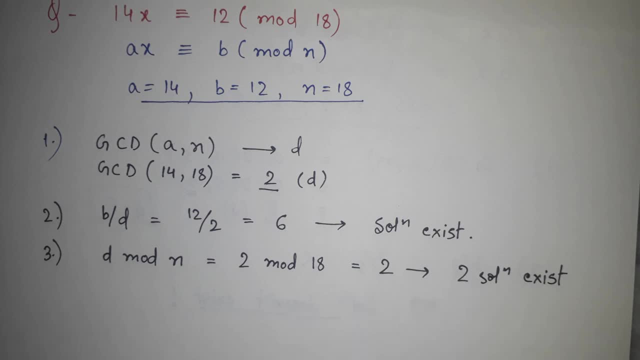 exist means at the end I will get two values of x right. So this is my third step. So I will get two values of x right. So this is my third step. So I will get two values of x right. So fourth step says that divide both the sides by d. Divide both the sides by d, Divide both the. 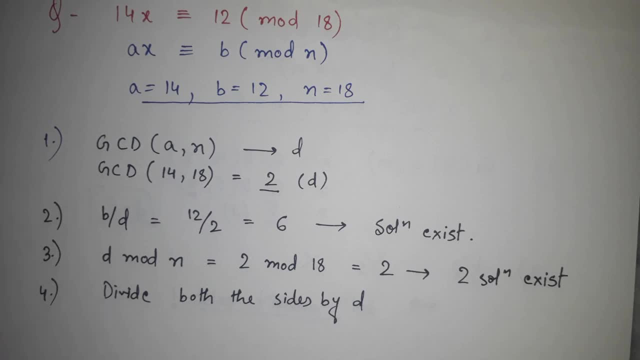 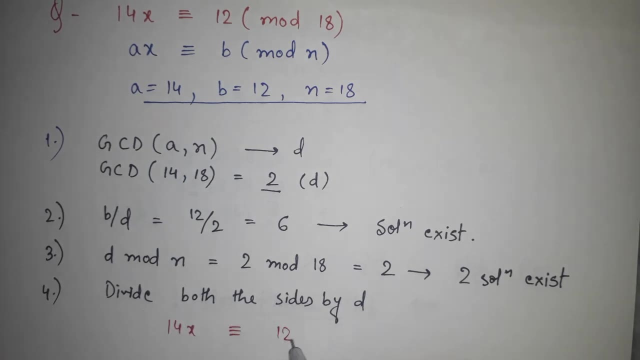 sides by d. So both the sides by d means by default. my equation is my equation that is already given, So it was 14x- is congruent to 12 mod 18. right Now, what we have to do is we have to. what I have to do is I have to divide both the sides by d. In my case d is 2.. So I will divide. 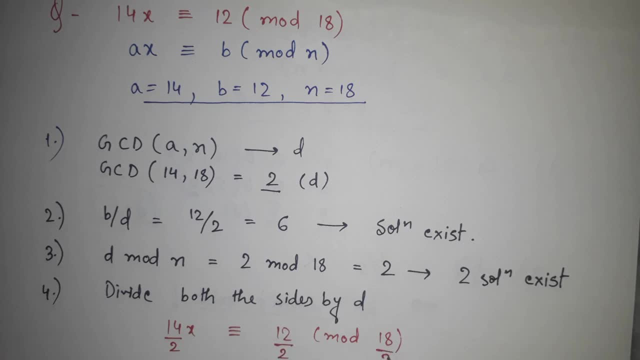 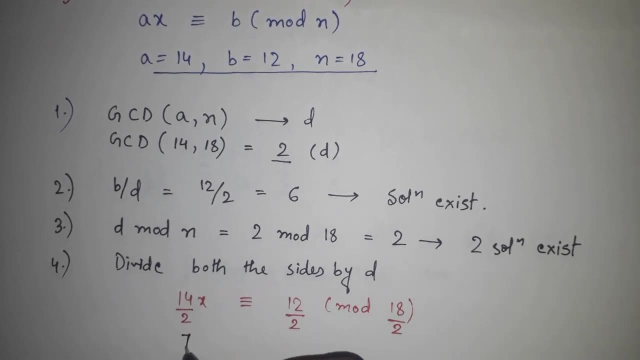 both the sides, all the numbers by 2.. So dividing them what I will get is dividing them, I will get. 7x is congruent to 6 mod 9, right, I will get this equation: that 7x. 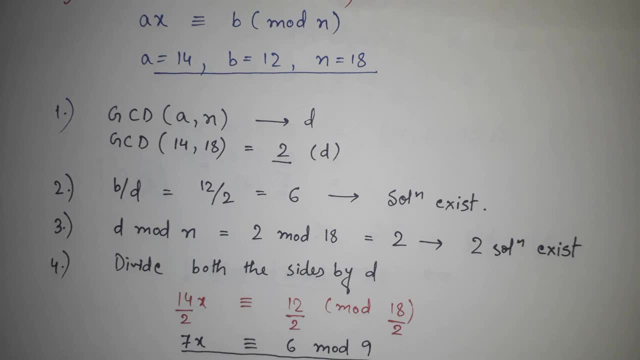 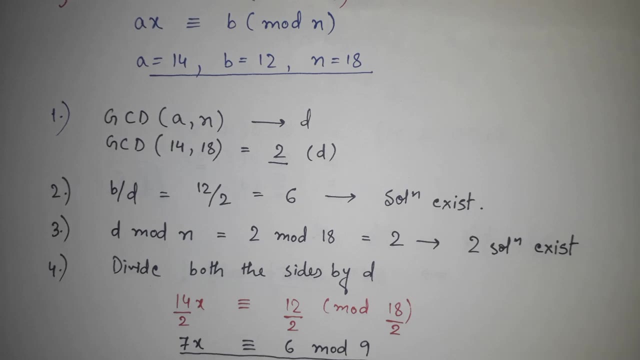 is congruent to 6, mod 9.. Now I have got this in the fourth step, So from the fifth step I will take this equation and I will carry out. This is my fourth step. Then in the fifth step: 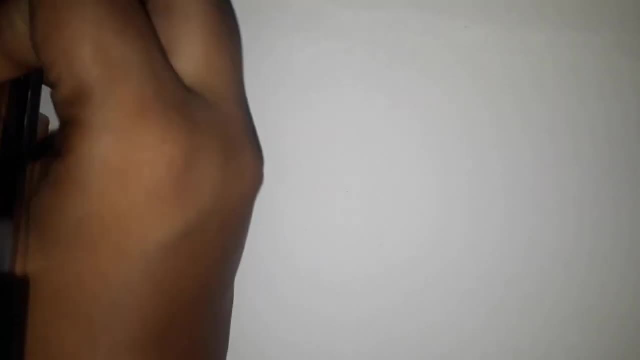 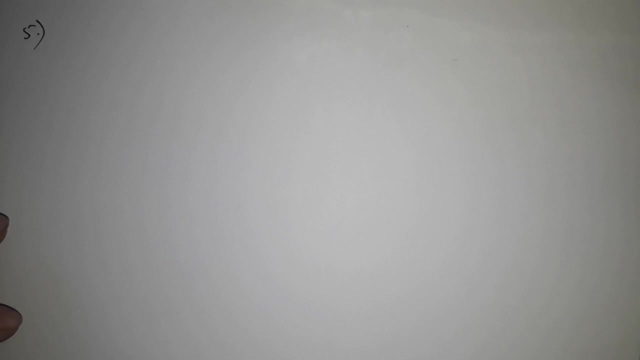 what I will do is in the fifth step. in the fifth step, I am having you take those steps, take those steps with you So you can get a clear idea, Though I am writing the steps, okay, from here here up to here, we have done up to the fourth step. 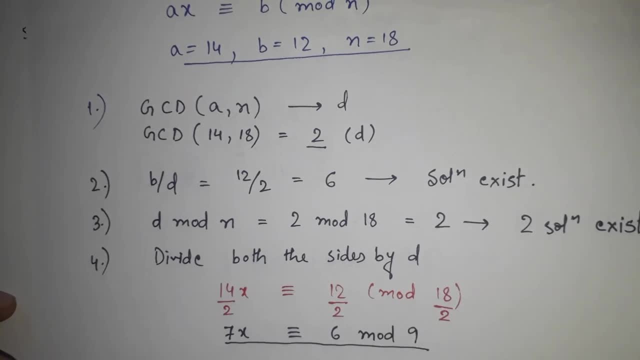 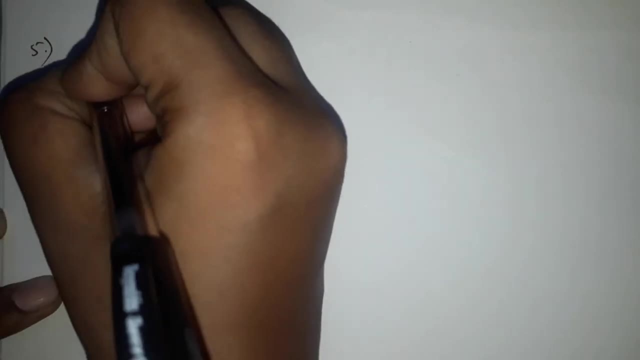 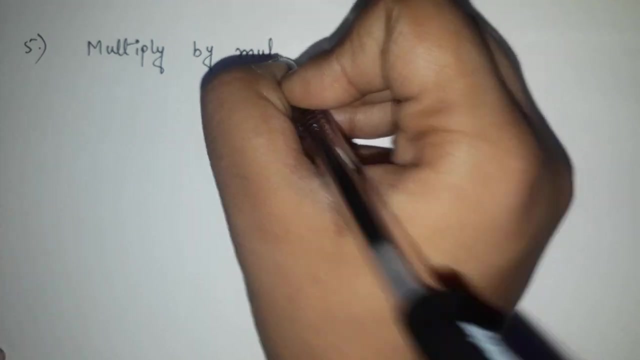 dividing both the sides by d. Okay, after dividing both the sides by d, what my fifth step would be? Multiply both the sides by multiplicative inverse of a. Multiply both the sides by multiplicative inverse of a, by multiplicative inverse of a right. 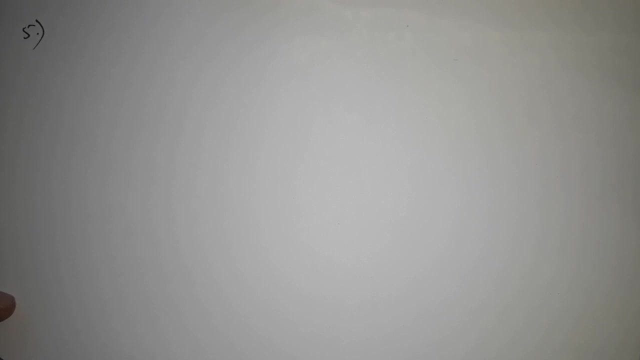 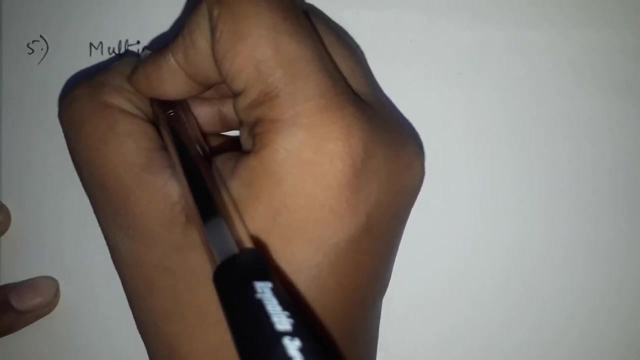 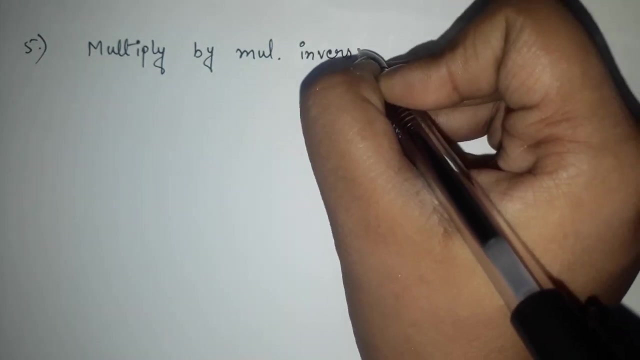 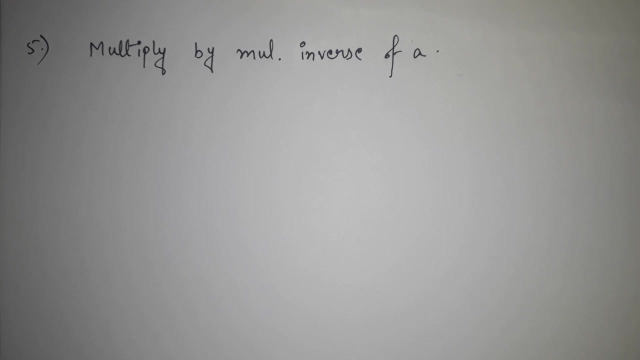 the sides by d what my fifth step would be. multiply both the sides by multiplicative inverse of a. multiply both the sides by multiplicative inverse of a. So the equation that we got in the previous step is: 7x is congruent to 6 mod 9, right. 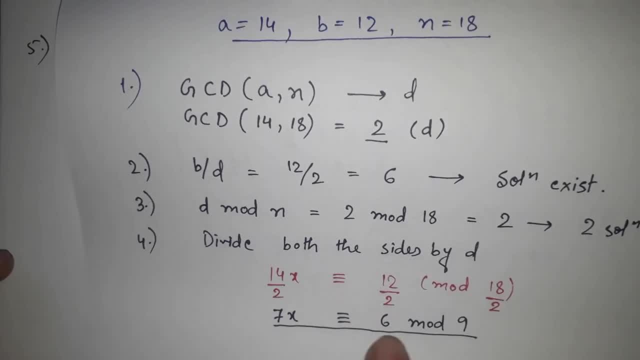 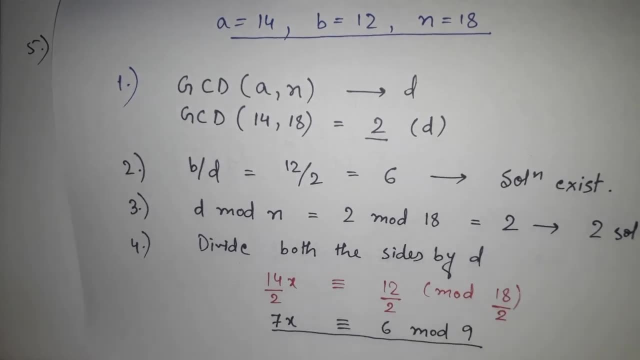 the equation that we have already found out, 7x is congruent to 6 mod 9, so we will multiply in this equation. we will multiply both the sides with A inverse, that is, 7 inverse. so because our A is 7.. 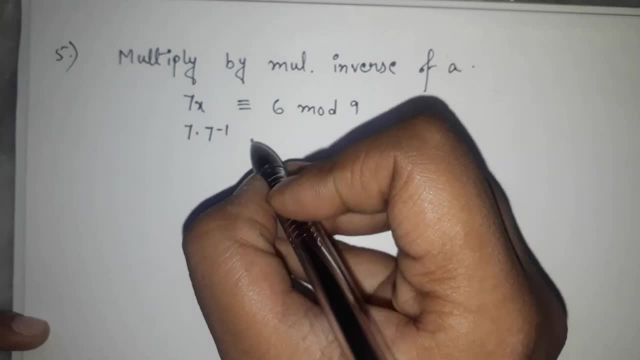 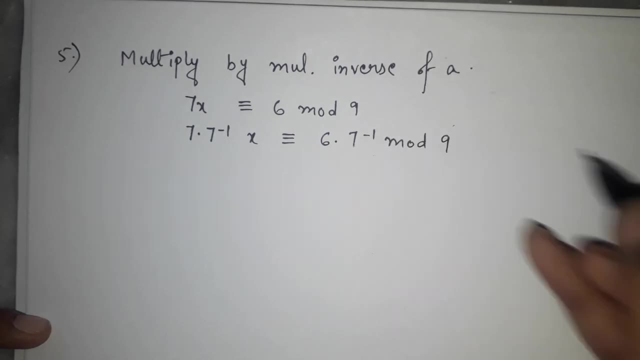 So what I will do is: 7 into 7 is 8.. So what I have done is I have taken the other side by 7 and I have taken both the sides. 7, inverse of X, is congruent to 6 into 7, inverse of mode 9.. What I have done, I have not done. 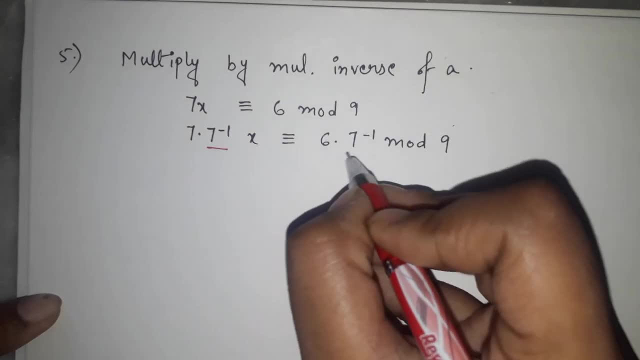 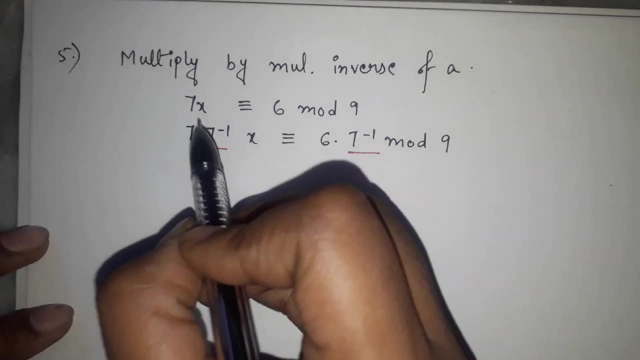 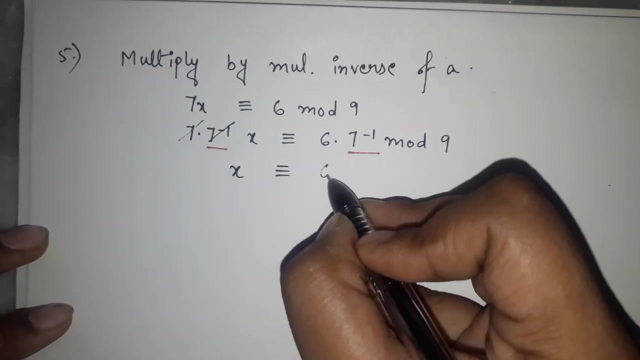 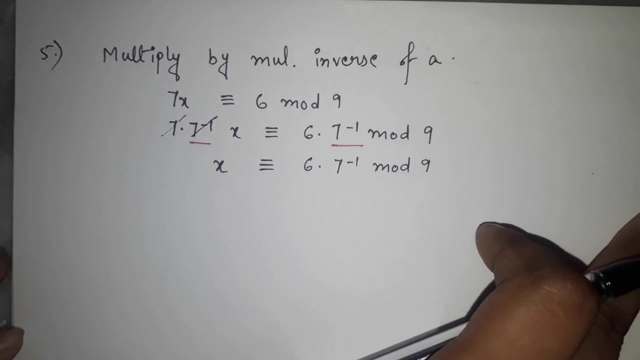 anything that big. I have just multiplied A inverse, that is 7 inverse, both the sides, right? So then here, as you know, 7, 7 inverse will get cancelled out. We will get only X. this side is congruent to Now. this is quite difficult to find. I will not say difficult If you are new. 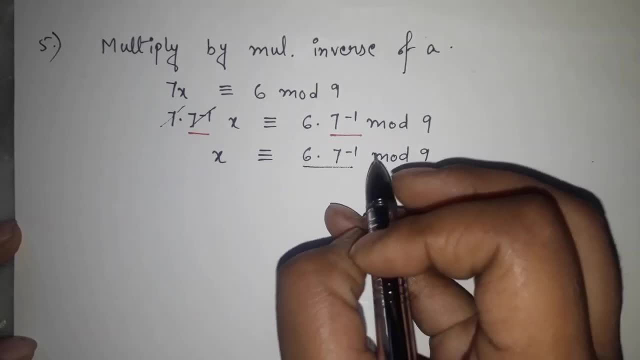 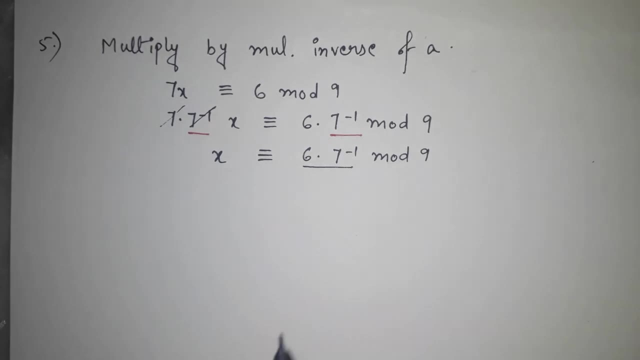 it will be difficult for you, But see, what we have to find is we have to find out the value of 7 inverse, and we will replace it here Now. how to find out the value of 7 inverse. I have already posted a video of how to find out the multiplicative inverse with the help of extended Euclidean. 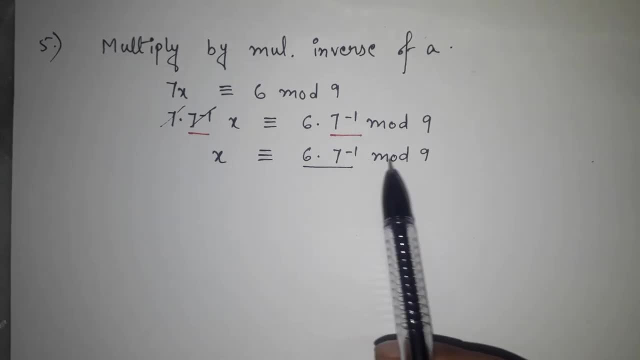 method. So that is one of the very good ways how you can find out this easily. Okay, like you won't get confused much, You can, with the help of that method finding- you can search my video on finding multiplicative inverse with the help of extended Euclidean method So you can get the 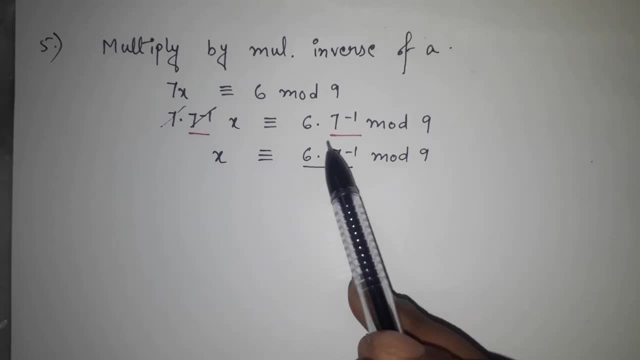 multiplicative inverse. So with the help of that method you can find the multiplicative inverse of 7 inverse. Apart from that, if I tell you a simple like quickly, how you can find out shortcut kind of thing, So how this can be interpreted. 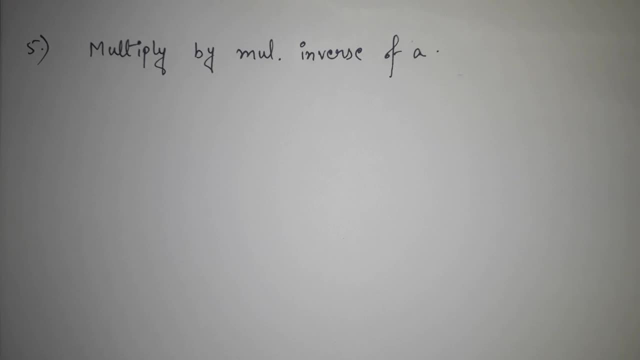 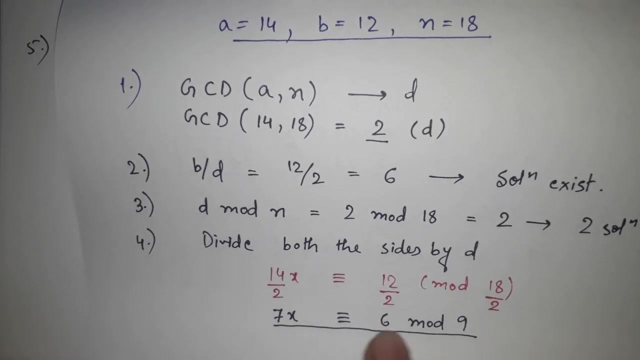 So the equation that we got in the previous step is: 7x is congruent to 6 mod 9, right, The equation that we have already found out: 7x is congruent to 6 mod 9.. So we will multiply in this equation. 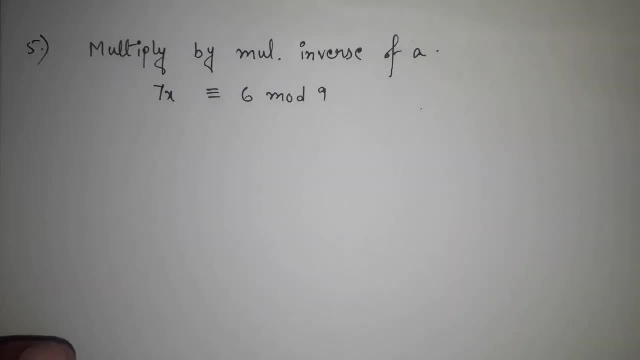 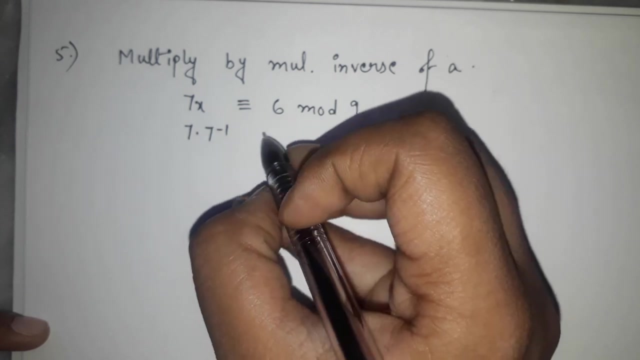 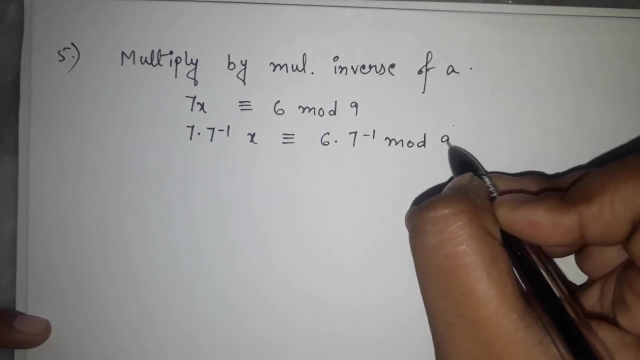 we will multiply both the sides with a inverse, that is, 7 inverse So, because our a is 7.. So what I will do is 7 into 7, inverse of x is congruent to 6 into 7, inverse of mod 9.. What I have done? I have not done anything that big. 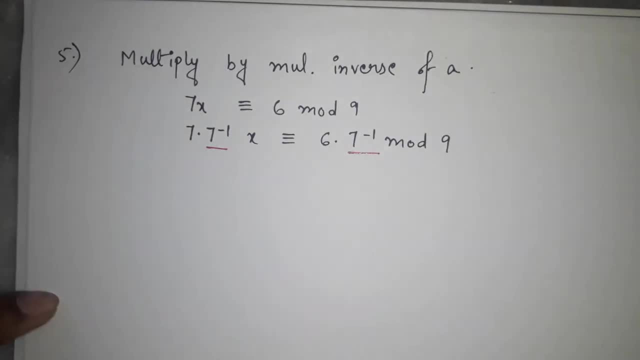 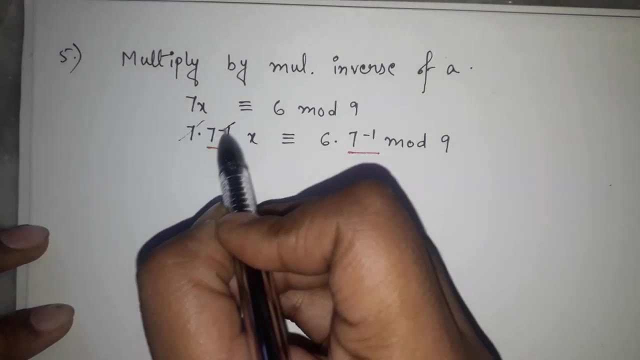 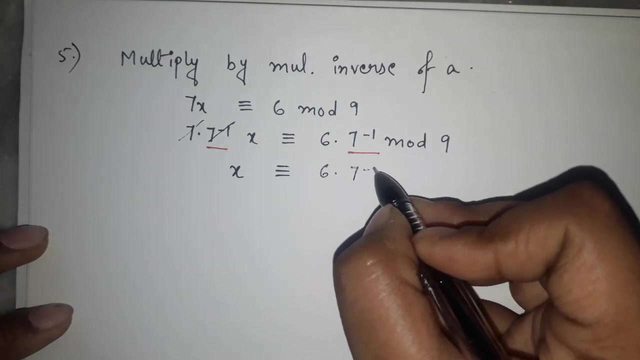 I have just multiplied a inverse, that is 7 inverse, both the sides, right. So then here, as you know, 7, 7 inverse will get cancelled out. We will get only x. this side is congruent to Now. this is quite difficult to find, I will not say difficult. 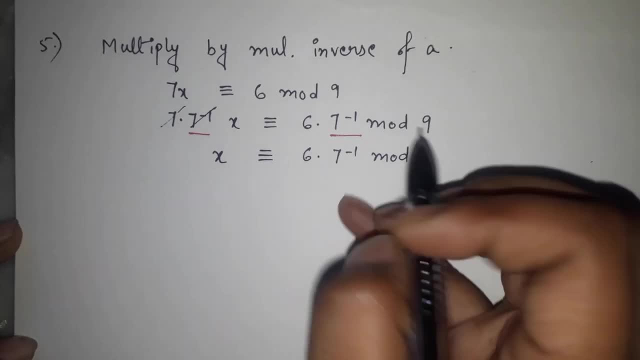 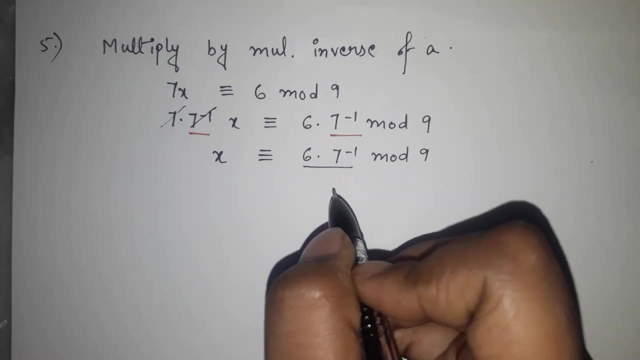 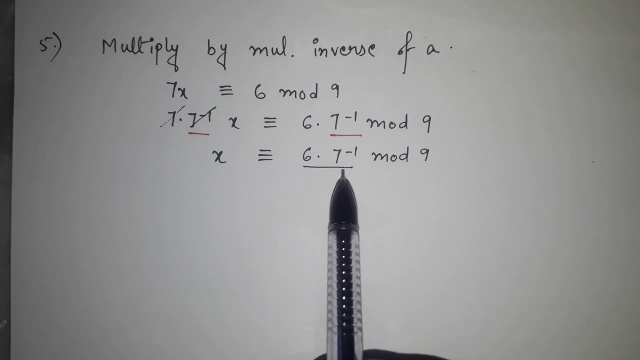 but if you are new it will be difficult for you. but see, what we have to find is we have to find out the value of 7 inverse and we will replace it here Now. how to find out the value of 7 inverse. I have already posted a video of how to find out the multiplicative. 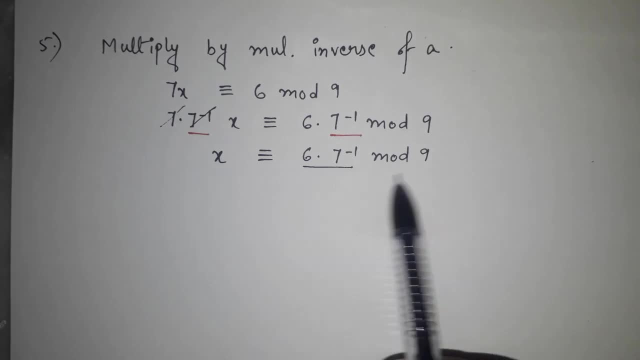 inverse with the help of extended Euclidean method. So that is one of the very good ways how you can find out this easily. okay, Like you won't get confused much, you can, with the help of that method, finding. 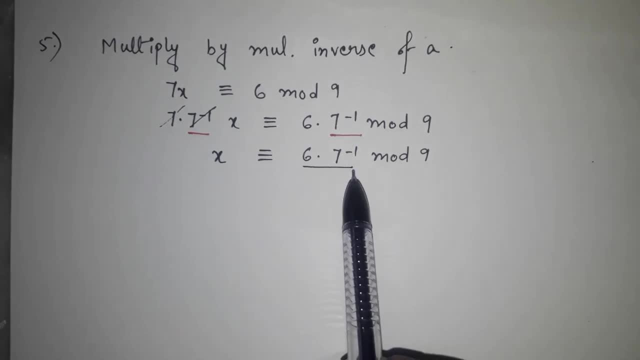 you can search my video on finding multiplicative inverse with the help of extended Euclidean method So you can get the multiplicative inverse. So with the help of that method you can find the multiplicative inverse of 7 inverse. Apart from that, if I tell you, 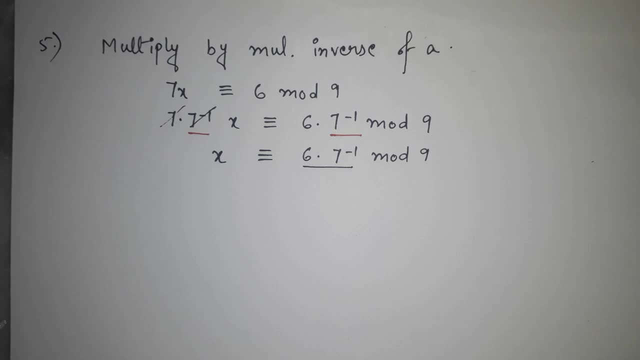 a simple like quickly, how you can find out shortcut, kind of thing. So how this can be interpreted. You can interpret this as 7 into anything like x mod n. Let's say 7 into x, so let's not here we are having x, so let's take it anything else like a, b or 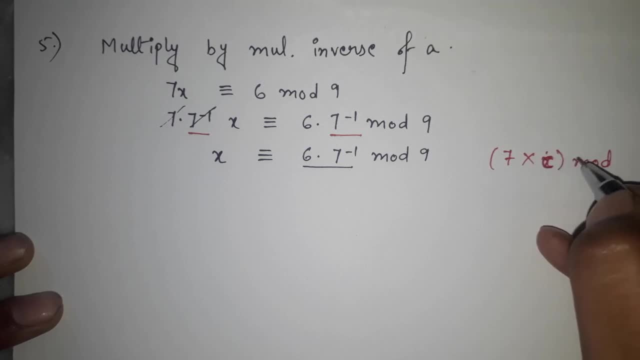 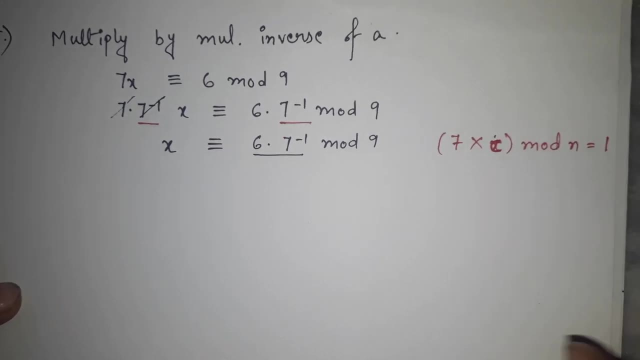 anything. Let's take it as c. okay. 7 into c, mod n. you should get this as 1, okay. You can interpret it like this: that 7 into c, 7 means because 7 inverse. we have to find. 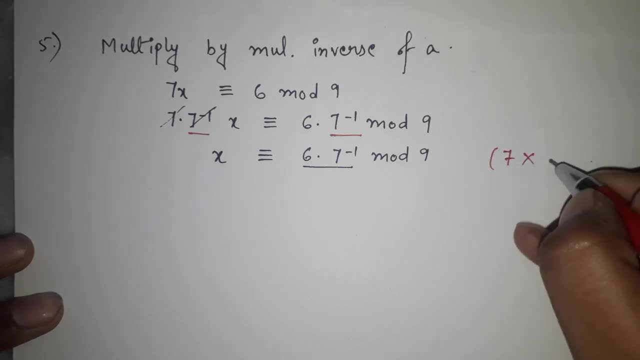 You can interpret this as 7 into anything like x mod n. Let's not here, we are having x, So let's take it anything else, like a, b or anything. Let's take it as c. Okay, 7 into c mod n. 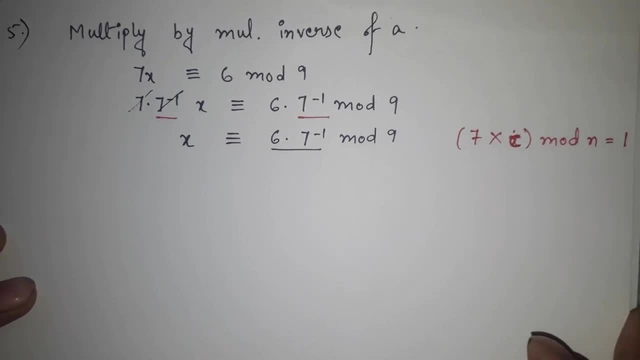 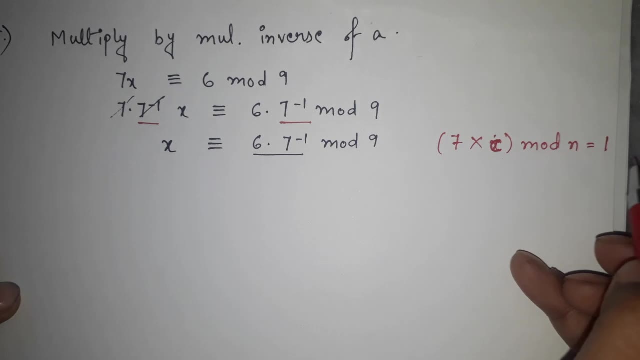 you should get this as 1.. Okay, you can interpret it like this, That's 7 into c. 7 means because 7 inverse. we have to find out. So 7 into c mod n should be equal to 1. So 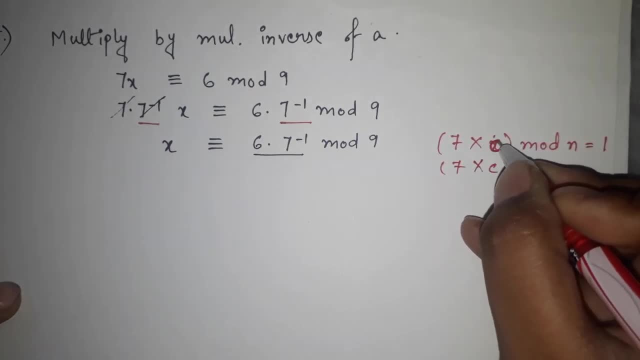 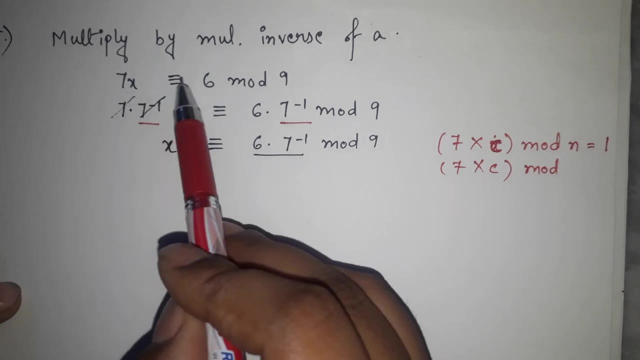 7 into c- This c is something c would be 7 inverse- That you have to find out, Mod, what the value of n is. as we know, this is ax congruent to b mod n. So in this case, 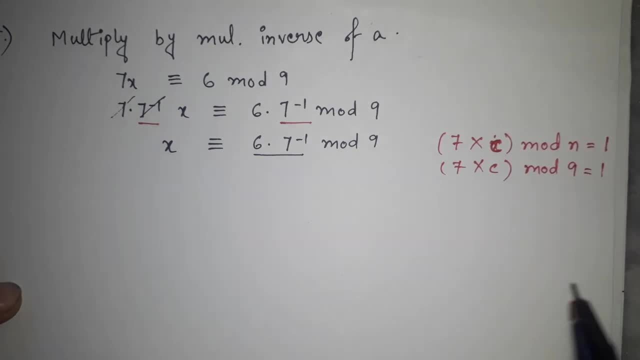 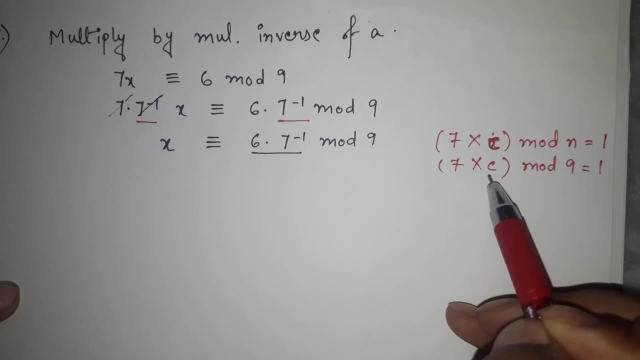 my n is 9 equal to 1.. So what I mean to say is: you have to find such a value of 7, that such a value of c that after multiplying this value with 7 and finding the mod of of 9, mod 9 on it, you will get the value 1.. Simple, You can simply use try and error One. 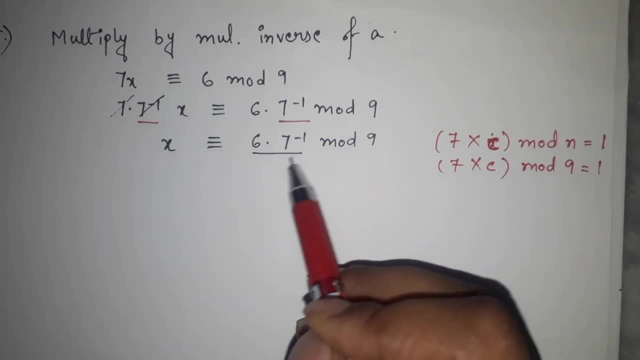 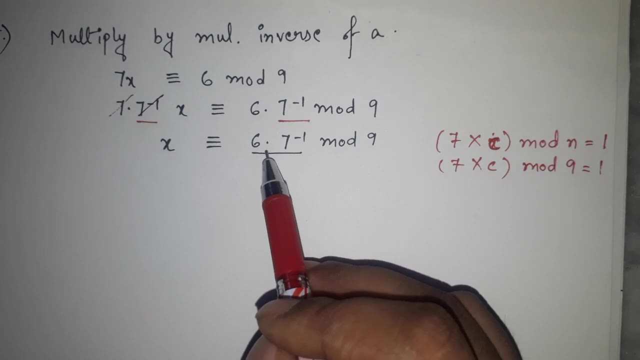 method, as I have already told. You can see that method or you can directly apply that method and get the answer. If you don't want to waste that much of time, it will take quite good amount of time. If you want to do it directly, you can do directly also. This is the method, how you can do. 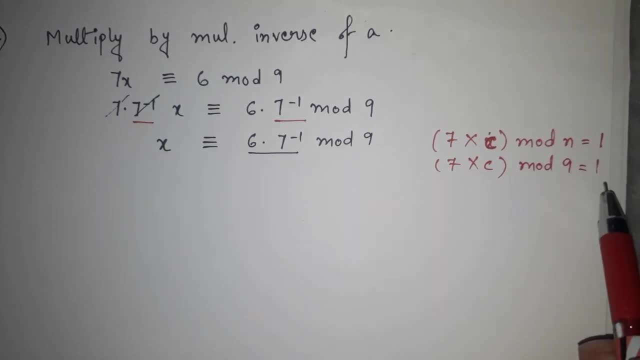 directly 7 into c mod 9, this mod 9 equal to 1, means we have to do kind of try and error and we will get a value of c such that after multiplying c with 7 and finding out mod n, we will get 1.. 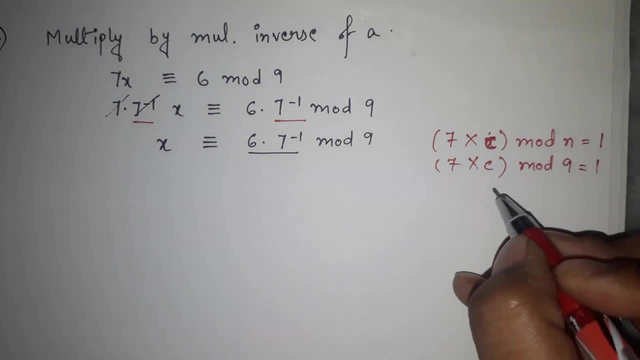 So if I see like let me show you how you can do, Let's take c equal to 1. If I am taking c equal to 1,, 7 into 1, that is equal to 7 mod 9.. 7 mod 9 will be equal to 7.. So it will not be equal to 1.. 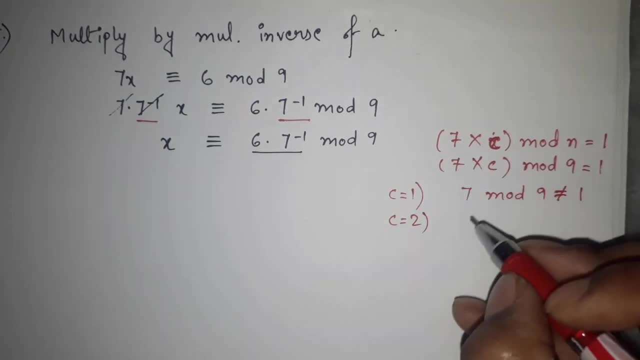 If I am taking c equal to 2,, 7 into 2 would be 14 mod 9 would be equal to 7 mod 9.. So c equal to 14 mod 9 will be equal to 5.. It is again not equal to 1.. I want something whose. 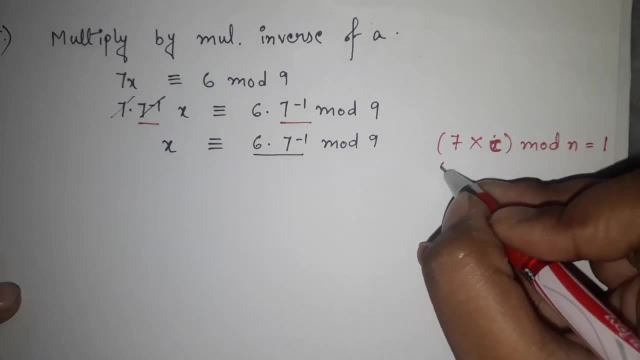 out. so 7 into c mod n should be equal to 1.. So 7 into c, this c, is something c would be 7 inverse that you have to find out. So 7 of n is, as we know this is ax- congruent to b mod n. So in this case my n is 9 equal. 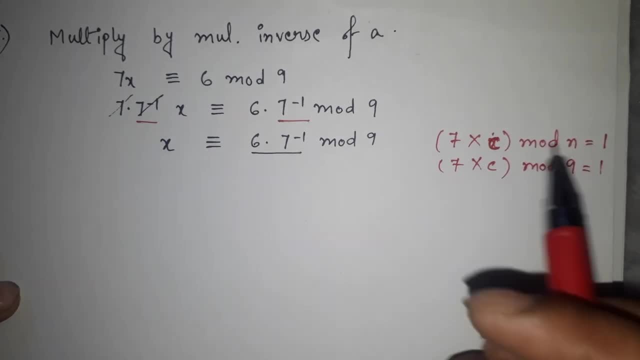 to 1.. So what I mean to say is: you have to find such a value of 7, that such a value of c that, after multiplying this value with 7 and finding the mod of 9,, mod 9 on it, you 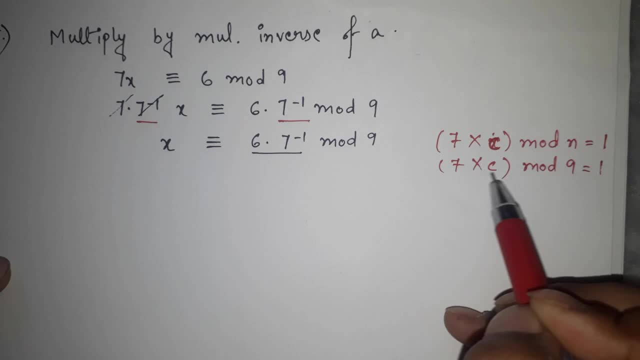 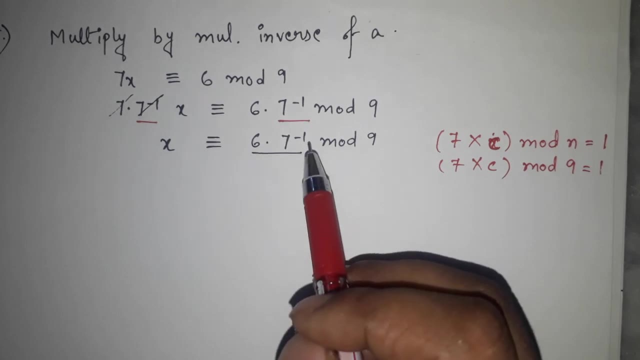 will get the value 1.. Simple: you can simply use try and error One method, as I have already told. you can see that method or you can directly apply that method and get the answer. If you don't want to waste that much of time, it will take quite good amount of time If you. 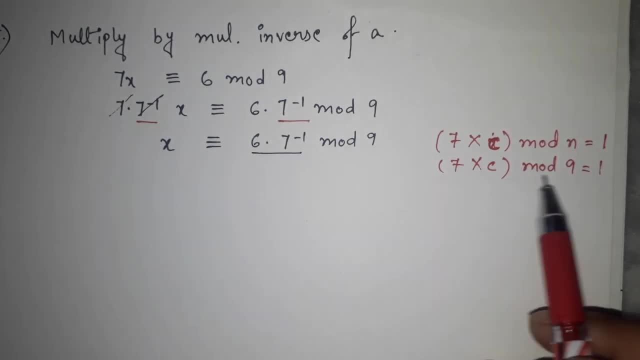 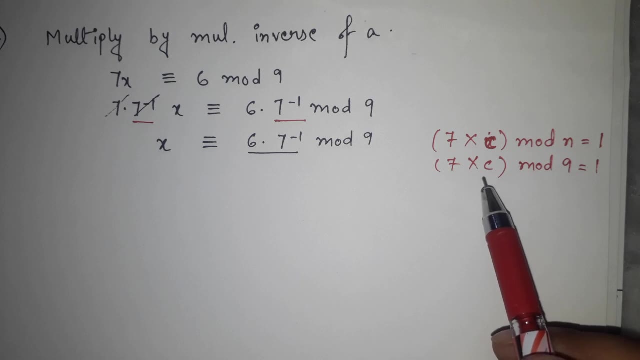 want to do it directly, you can do directly also. This is the method, how you can do directly 7 into c mod 9, this mod 9, equal to 1, means we have to do kind of try and error and we 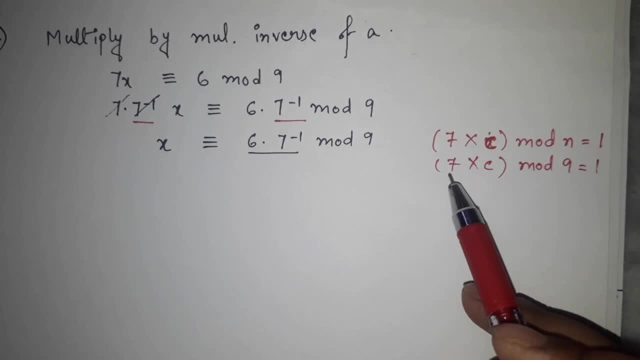 have to find a value of c such that after multiplying c with 7 and finding out mod n, we will get 1.. So if I see like, let's see, Let me show you how you can do, Let's take c equal to 1.. If I am taking c equal to 1,, 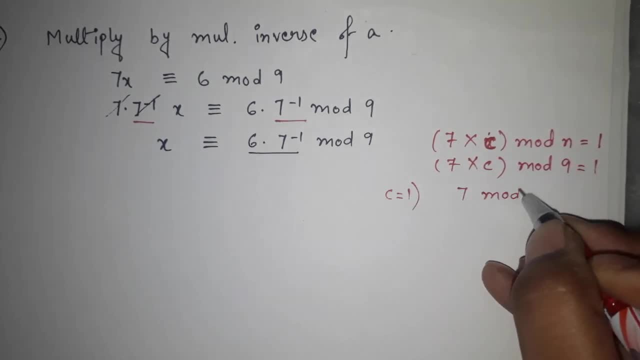 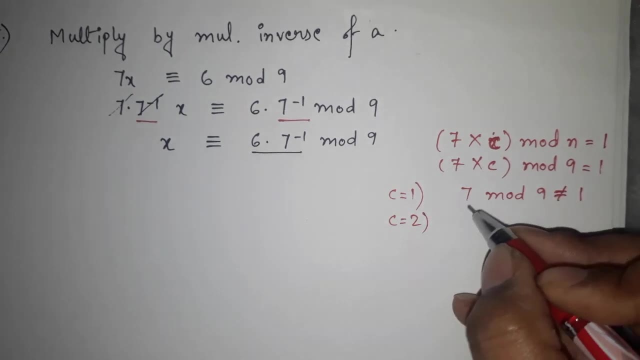 7 into 1, that is equal to 7 mod 9.. 7 mod 9 will be equal to 7.. So it will not be equal to 1.. If I am taking c equal to 2,, 7 into 2 would be 14.. Mod 9 would be equal to 14. 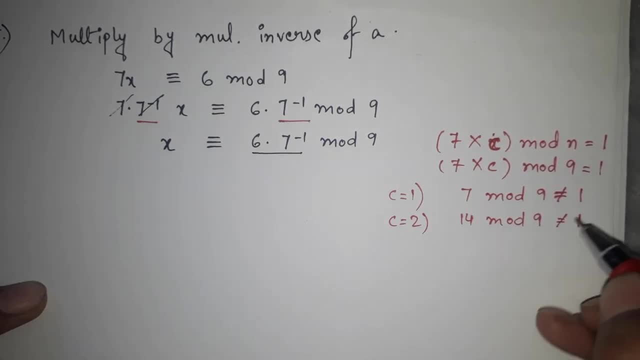 mod 9 will be equal to 5.. It is again not equal to 1.. I want something whose mod will be equal to 1.. So if I am taking c equal to 1,, I am taking c equal to 1.. So if I am. 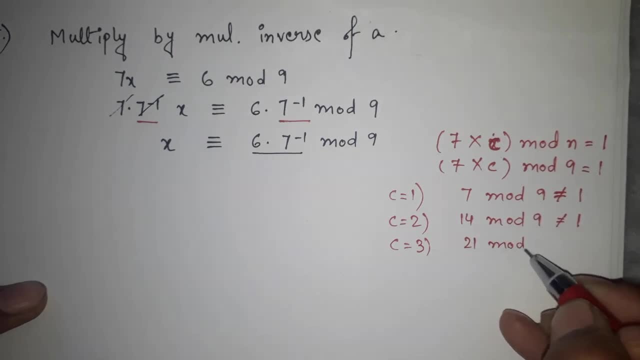 taking c equal to 3,, 7 into 3, equal to 21.. Mod 9,, the value will be 3,, which is again not equal to 1.. If I am taking c equal to 4, 7 into 4, equal to 28.. Mod 9,: 28 mod 9,. 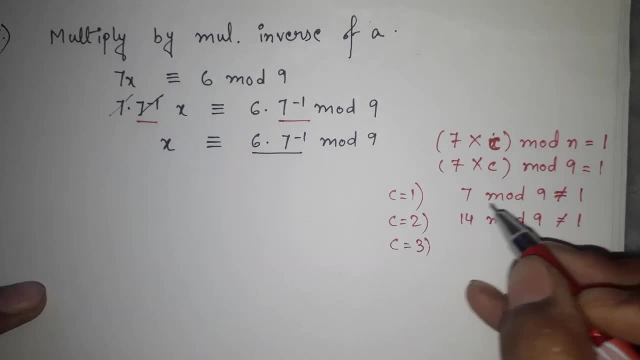 mod will be equal to 1.. So if I am taking c equal to 3, 7 into 3, equal to 21 mod 9, the value will be 3, which is again not equal to 1.. If I am taking c equal to 4, 7 into 4, equal to 28 mod 9, 28 mod. 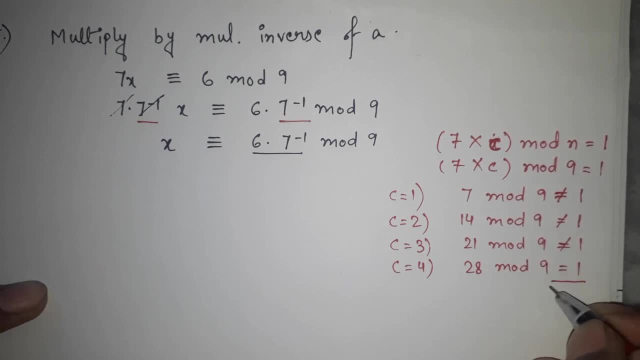 9, I will get 1.. So now, this is something where I am getting equal to 1.. So here, in this case, I am getting equal to 1, and my condition was I have to get equal to 1.. So here I am getting. 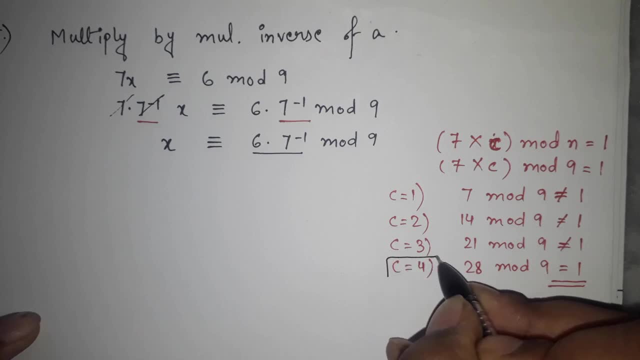 equal to 1.. So I can say that this case, this is c, like right, So this is c. This is my valid c, for which I am getting what I want. I am getting this multiplication mod 9, mod n, equal to 1.. I am. 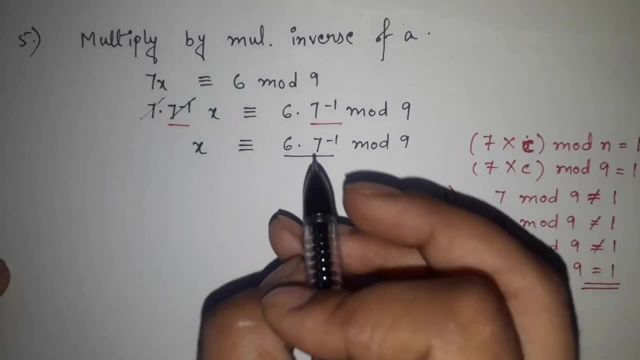 getting 1.. So I can say that c equal to 4 is correct. So what c equal to 4 is, c is, as I have told, 7 inverse. So what I will do is: I am getting 1.. So I am getting 1.. So I am getting 1.. So I. 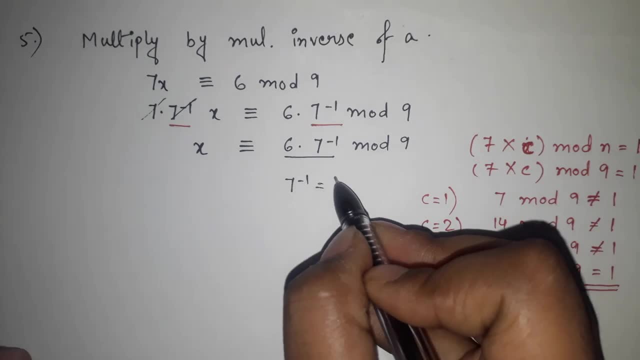 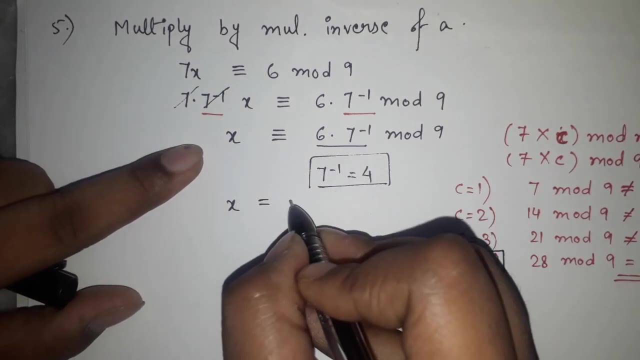 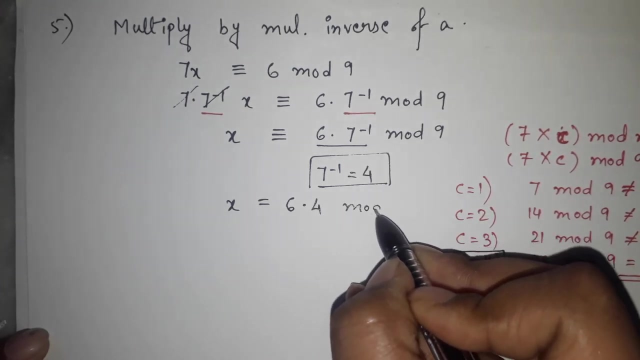 will replace this 7 inverse with my value 4.. Simple. So what it will become? x will be equal to. from here, x will be equal to 6 into 7 inverse. In place of 7 inverse, I will write 4 mod 9.. So 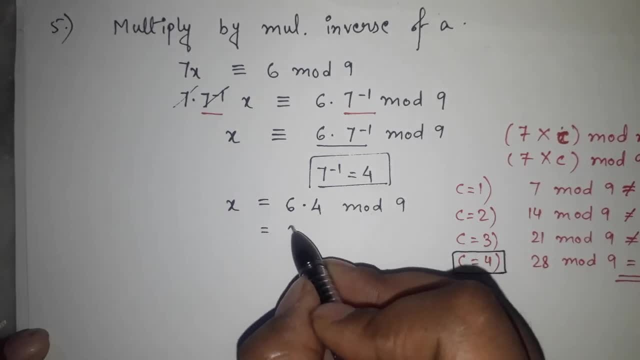 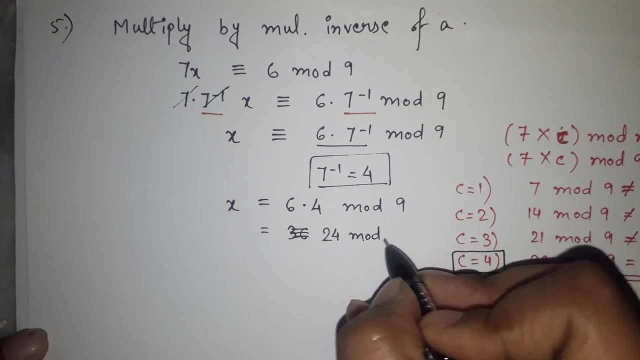 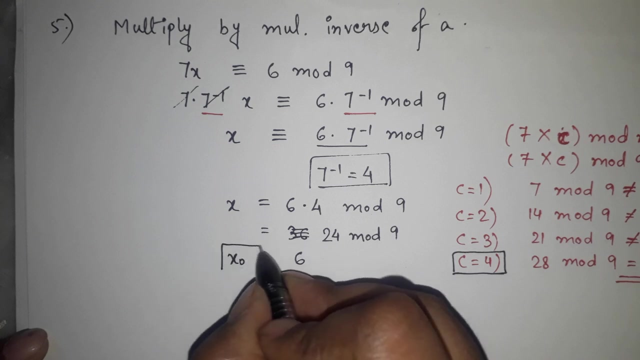 that is equal to 6 into 4, right 36.. 6 into 4 is 24 mod 9.. 24 mod 9, equal to 6.. So this is the first value of x that we have got Because, as we know, our 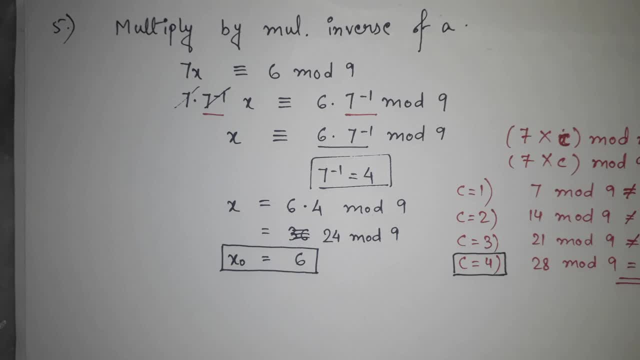 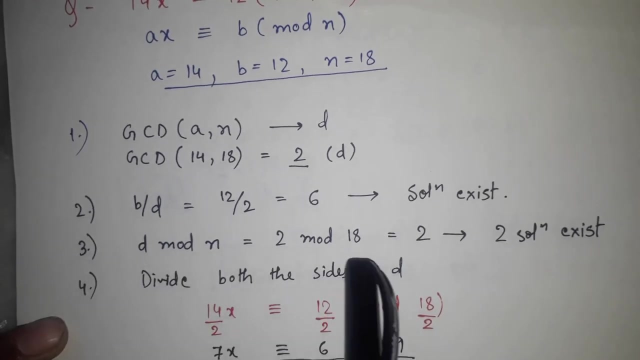 ultimate, our ultimate. the question is finding x or finding the value of x, the solution, So one solution that we got is x: 0 equal to 6.. What I told is here: see in the second step, what we in the third step, what we have found out, that 2, 2 means d mod n. we got 2.. 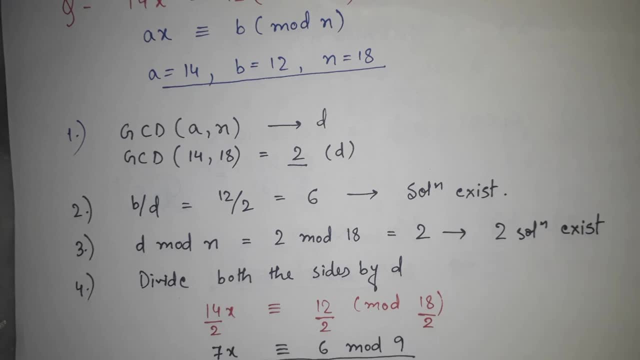 That means we have got x 0 equal to 6.. So we have got x 0 equal to 6.. So we have got x 0 equal to 6.. That means two solution exist. Two solution exist means I have told you in that step that we will. 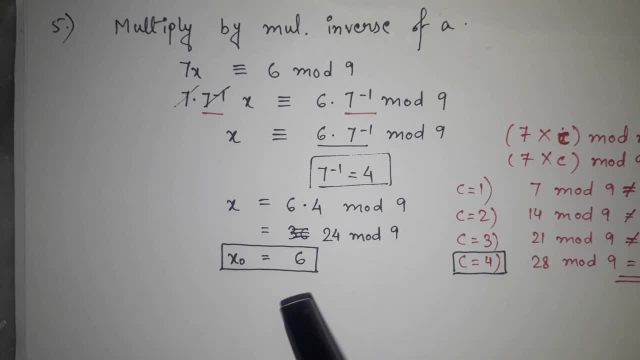 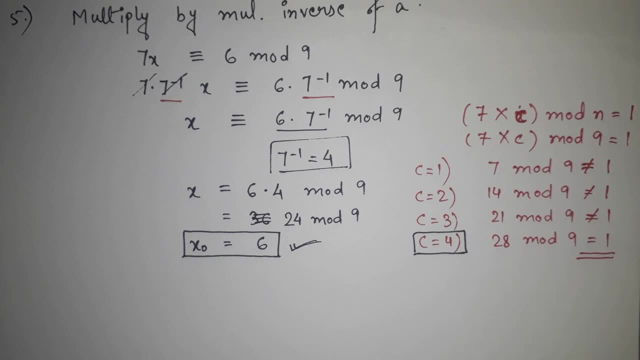 get two values of x. So x 0 equal to 6 means already one value. we got x 0 equal to 6 that we wanted right Now our last step is to find out second value of x. One value of x we already found. 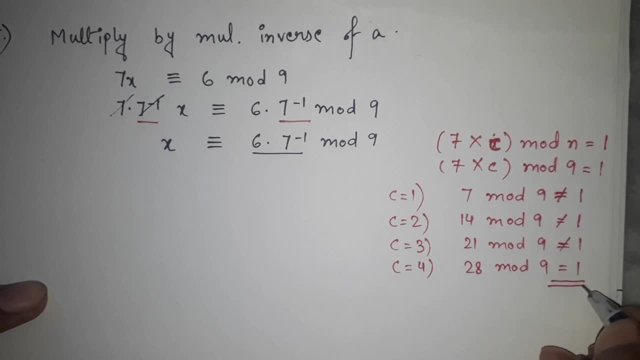 I will get 1.. Yes, So now this is something where I am getting equal to 1.. You are getting right. So here, in this case, I am getting equal to 1, and my condition was: I have to. 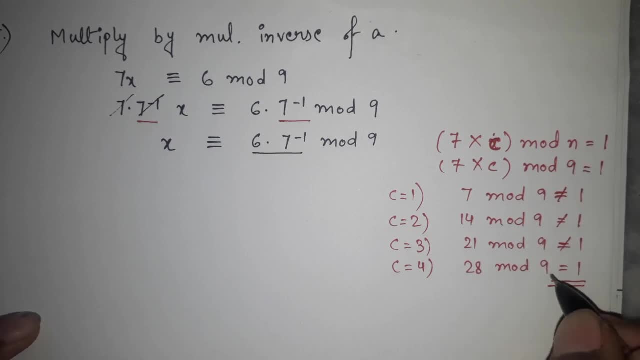 get equal to 1.. So here I am getting equal to 1.. So I can say that this case, this is c equal to 1.. So I am getting equal to 1.. So I am getting equal to 1.. So I am getting. 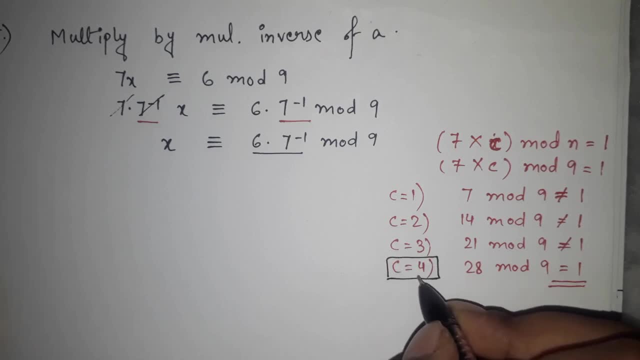 like right. So this is c, This is my valid c, for which I am getting what I want. I am getting this multiplication, mod 9, mod n equal to 1.. I am getting 1.. So I can say that c. 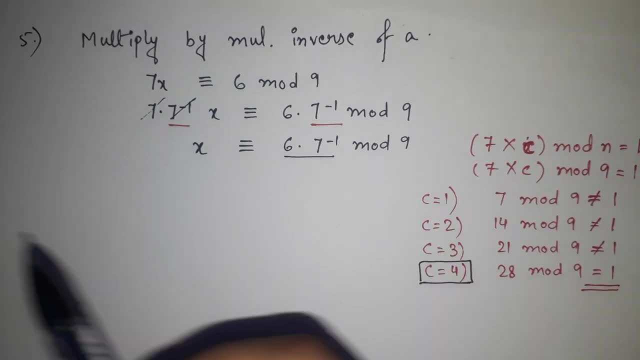 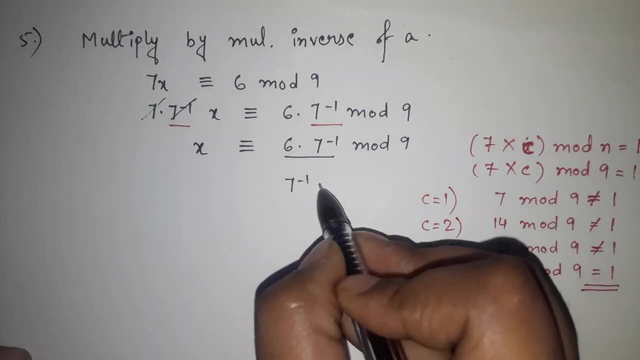 equal to 4 is correct. So what c equal to 4 is, c is, as I have told, 7 inverse. So what I will do is I will replace this 7 inverse with my value 4.. Simple, So what it will. 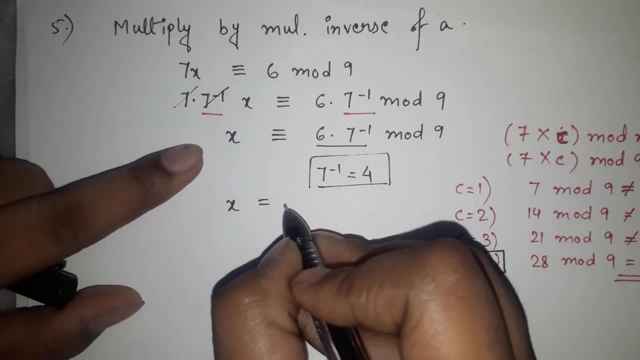 become, x will be equal to 7.. So what I will do is I will replace this 7 inverse with my value 4.. So what it will become x will be equal to. from here, x will be equal. 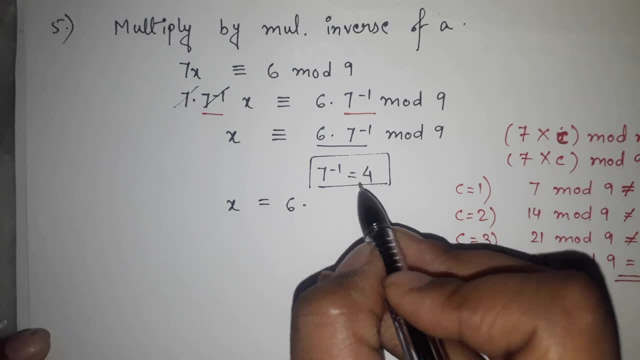 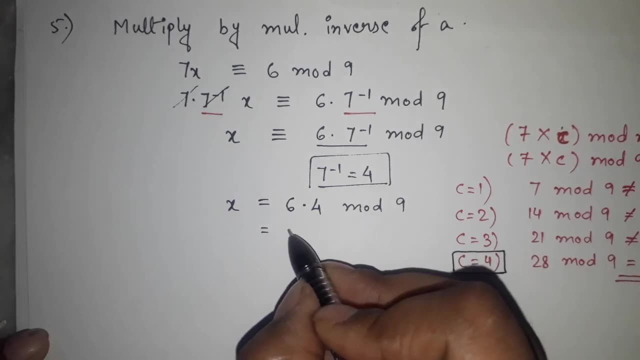 to 6 into 7 inverse. In place of 7 inverse, I will write 4 mod 9.. So that is equal to 6 into 4, right 36.. 6 for the 24.. 6 into 4 is 24 mod 9.. 24 mod 9 equal to 6.. So this: 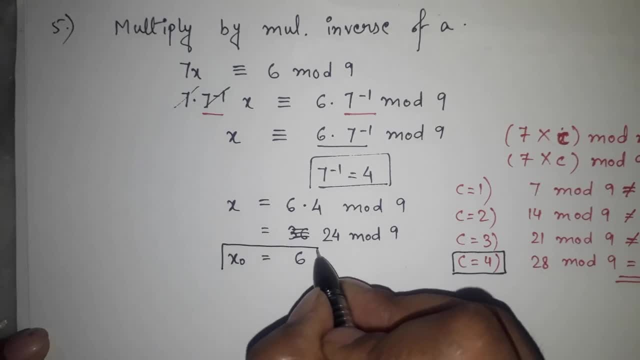 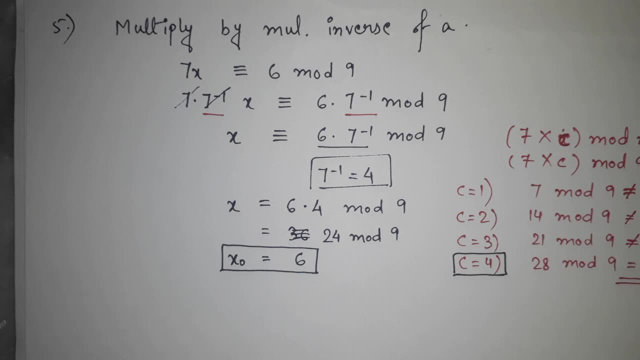 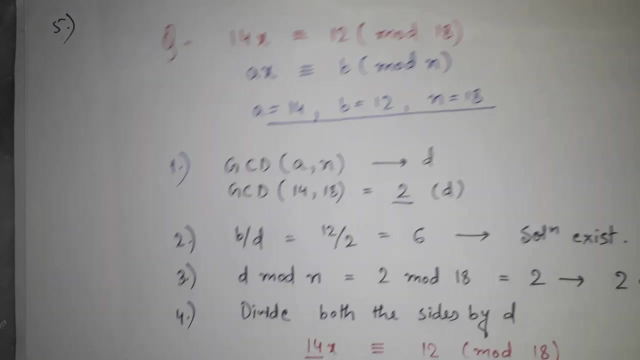 is the first value of x that we have got. We because, as we know our ultimate, we have our ultimate, our ultimate. the question is finding x or finding the value of x. the solution, So one solution that we got is x: 0 equal to 6.. What I told is here: see in: 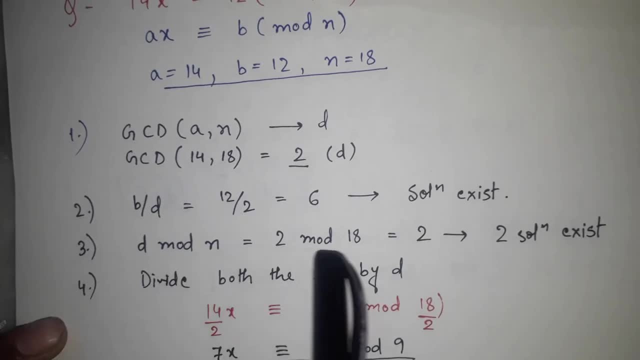 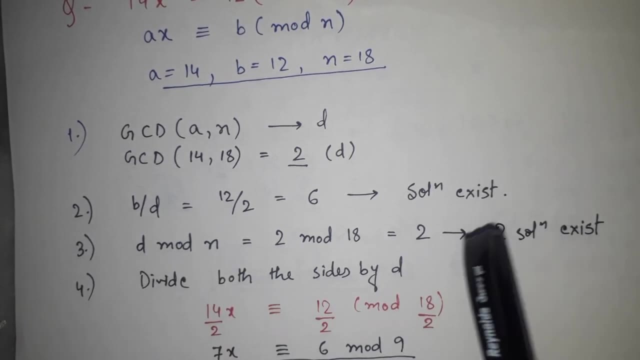 the second step, what we in the third step, what we have found out? that 2,, 2 means d mod n. we got 2.. That means 2 solution exist. 2 solution exist means, I have told you in: 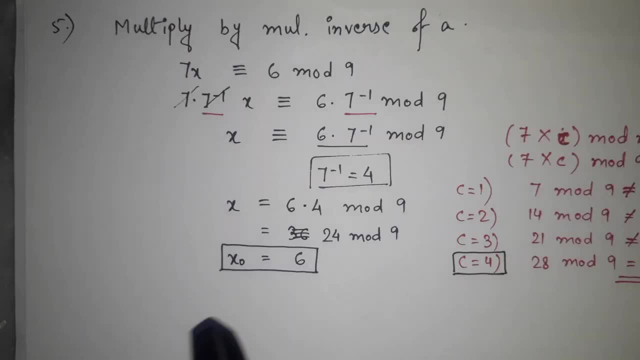 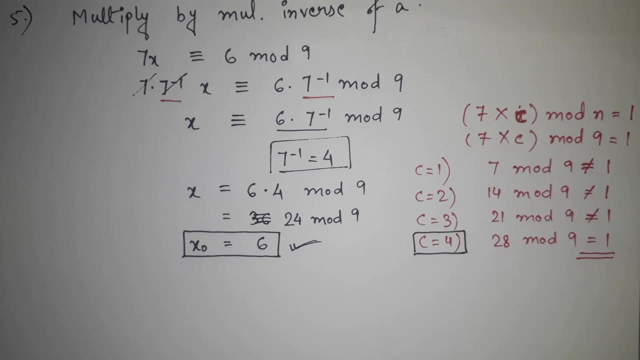 that step that we will get 2 values of x, So x 0 equal to 6.. So we have got x 0 equal to 6.. Means already one value. we got x 0 equal to 6 that we wanted right Now our last. 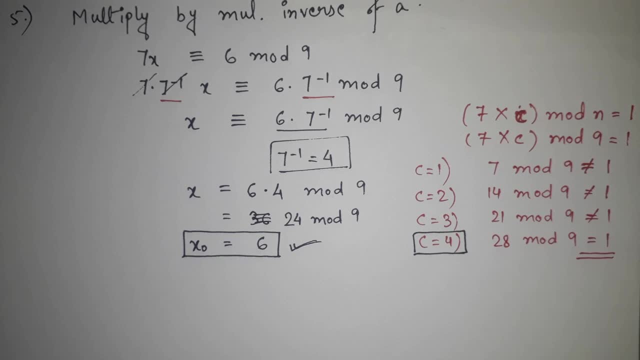 step is to find out second value of x, One value of x. we already found out Now second value of x. How we can find second value of x In the equation in the steps that we have discussed. The general equation of finding x is x, k equal to x, 0 plus k into n by d. 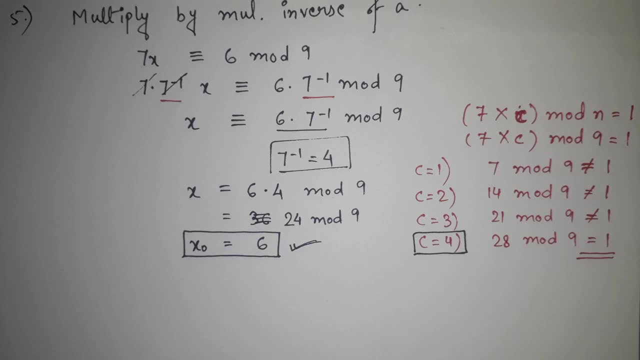 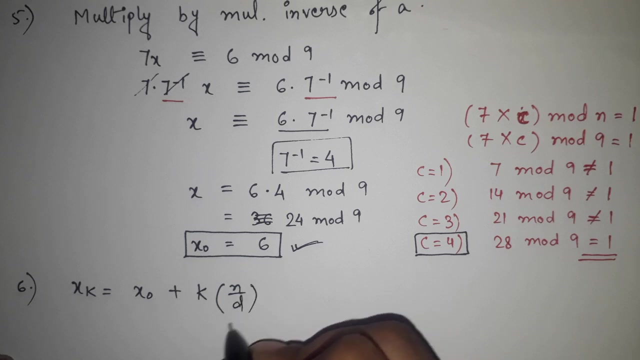 out Now second value of x. How we can find second value of x In the equation in the steps that we have discussed. The general equation of finding x is x k equal to x, 0 plus k into n by d. This was the general step of finding x. So here in this step, x 0,. 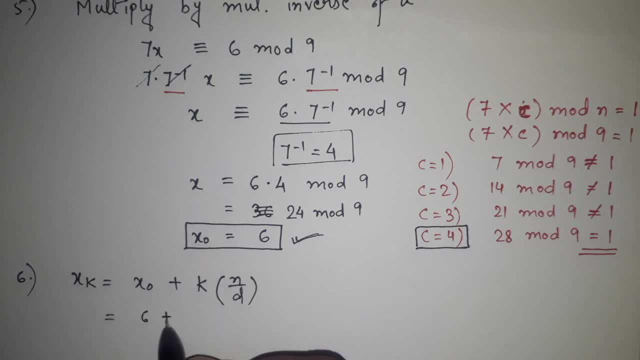 we are already having x 0, that is 6 plus k. What we will take k By default, we will take k as 1, 2, 3.. See, this is k. Now 1 x 0 we got. The second one will be x 1, right. 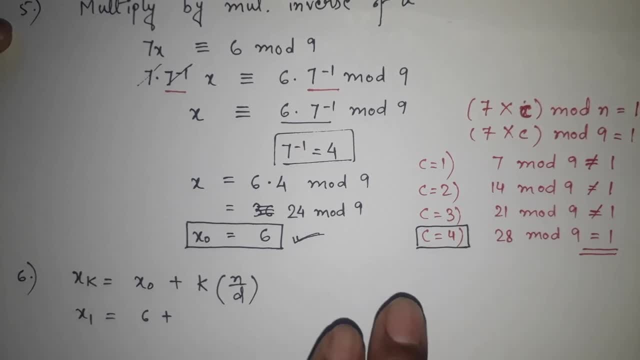 We know that we have two solutions possible in this question. In this, in case we were having three solutions, We have two solutions possible in this question. In this, in case we were having three solutions, Then we will get x 0,, x 1,, x 2.. But in this case only two solutions are. 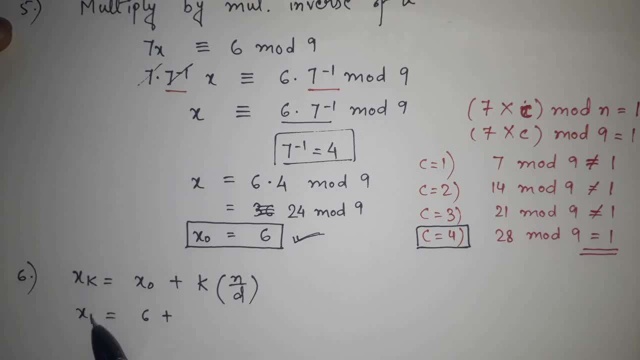 possible. So we will get x 0 and x 1.. So if this is 1,, this is k, as you can see. So this k will also be equal to 1.. Then n divided by t. In our case, in our question question what we were. 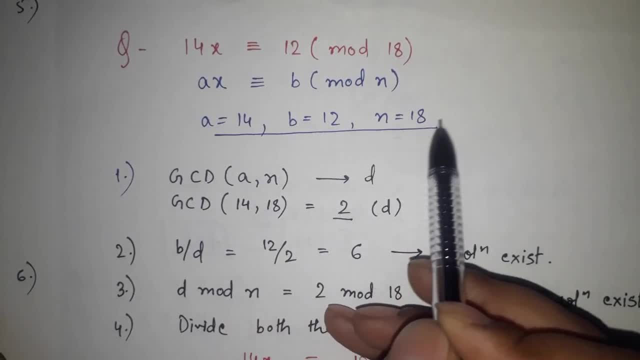 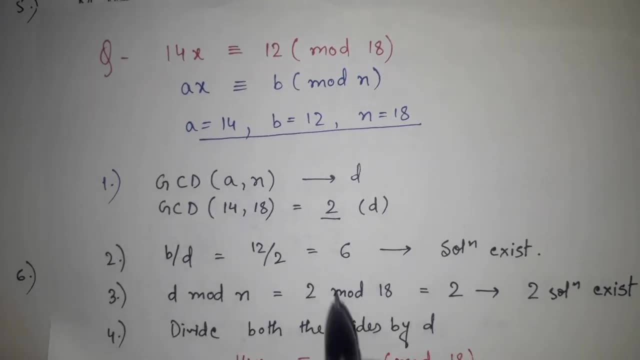 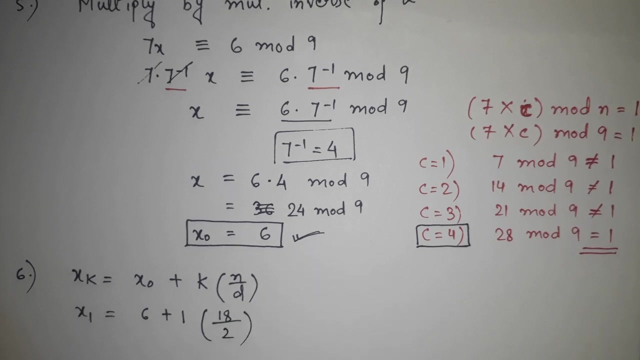 having a b? n. So n was equal to 18.. So n we have to take 18 and d in our question. d was d we have found out as 2, right d equal to 2.. So here we will get 2.. Simple, So x1. this is: 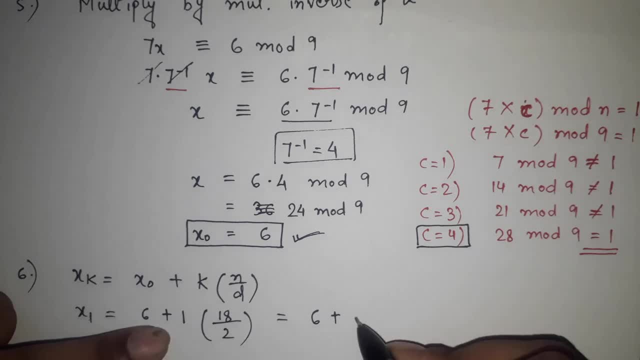 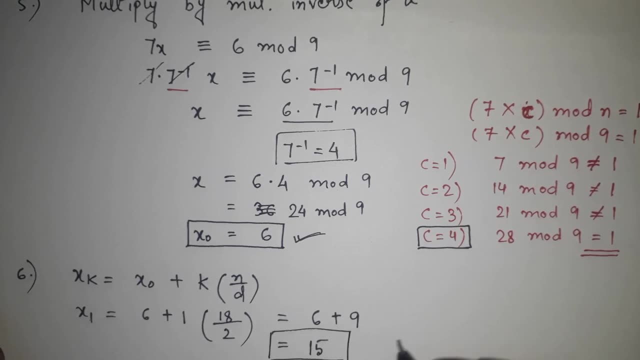 equal to 6 plus 1 into 18, divided by 2 is 9, that is equal to 15.. So you can say that x1 equal to 15.. So two solutions are possible. One of them is x0 equal to 6.. The second one is x1 equal to. 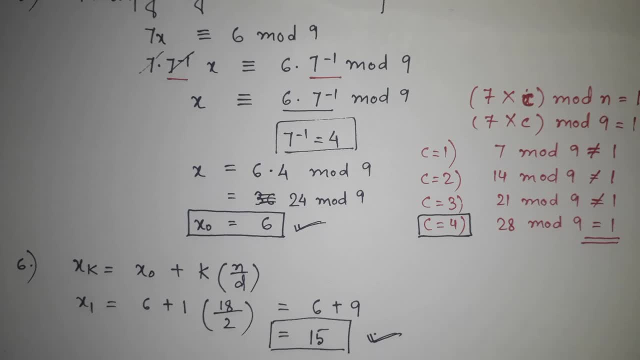 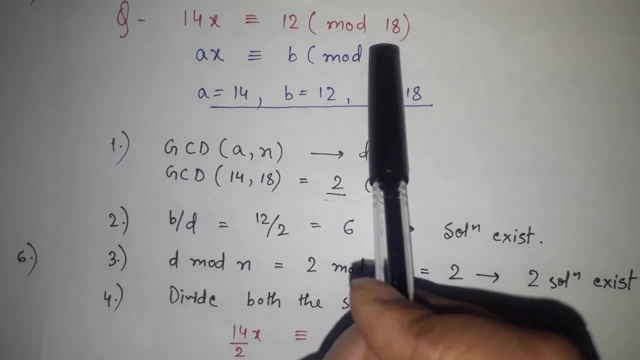 15.. So x and 15 are two values of x that we have found out. These are the two solutions. 6 and 15 are the two solutions of this particular question that we have solved, okay. So this is an example. 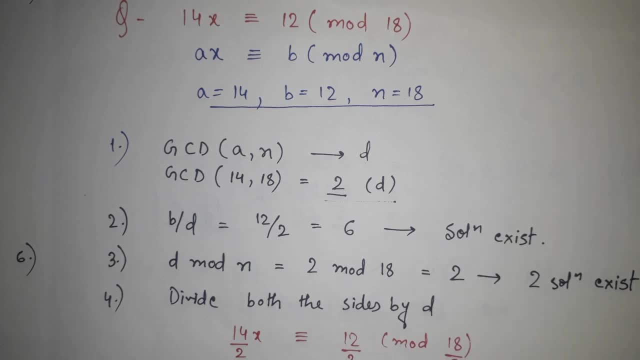 that I have taken In this example. almost all the steps are covered in detail. All the techniques are covered in detail. I have shown you how to find multiplicative inverse, the shortcut to find multiplicative inverse right. I hope you have understood all the steps. In case you still have, 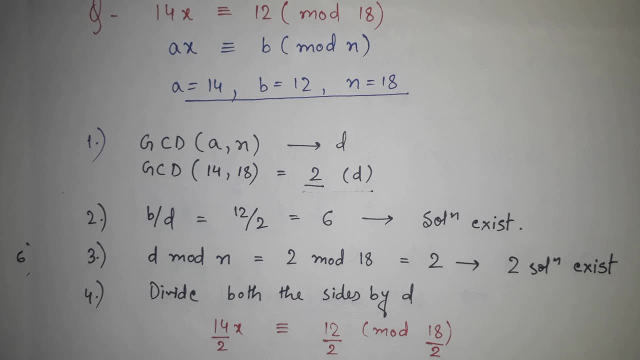 any doubt or you are stuck somewhere? please do not forget to subscribe to my channel, Thank you. Please ask us in the comment section. I will try my best to help you out. Thank you.